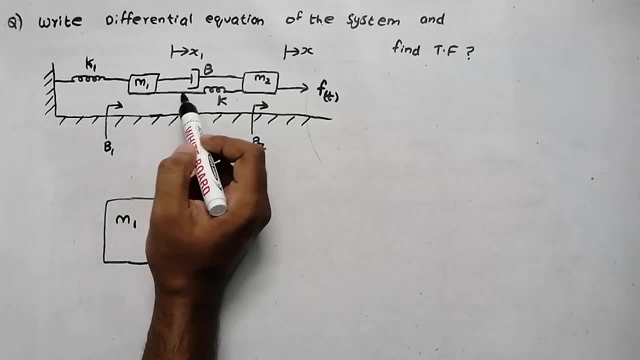 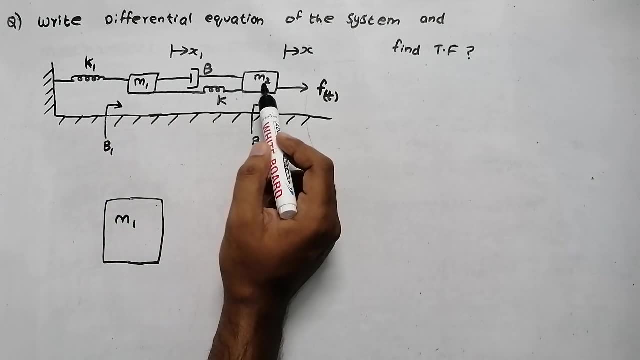 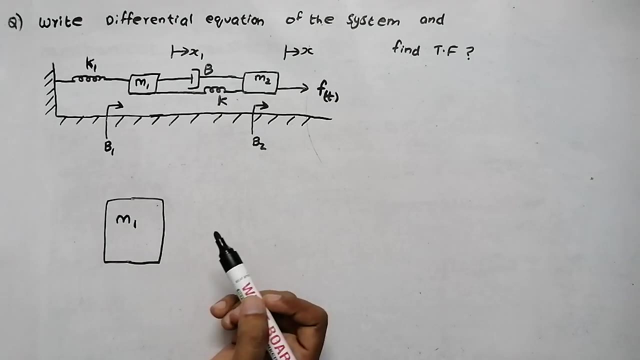 Here there is spring. Here there is dashboard. Here there is spring. Here there is dashboard. There are no applied forces around this mass m1. But as you can see in mass m2, here there is an applied force. So for mass m2 there is an applied force. For mass m1, there are no applied force. 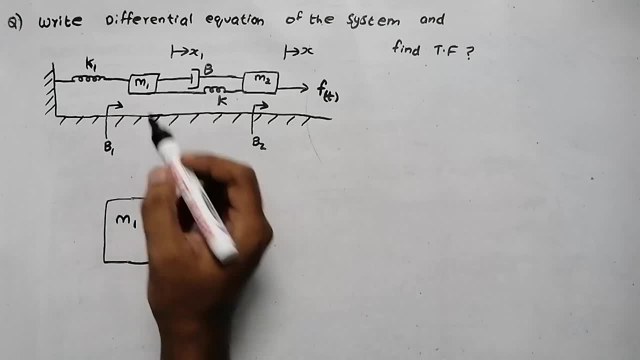 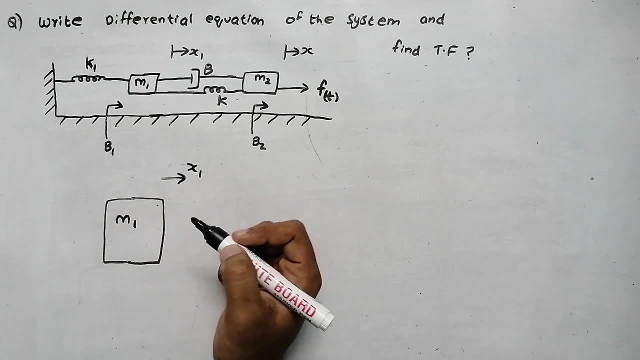 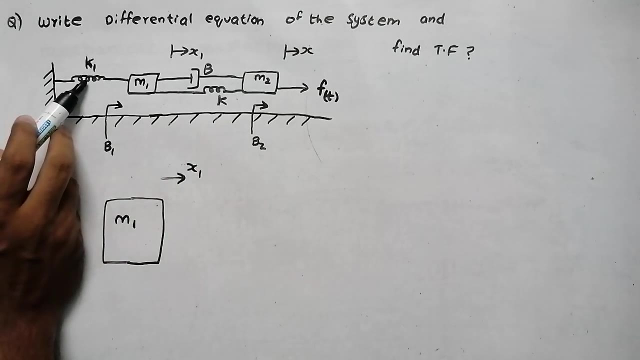 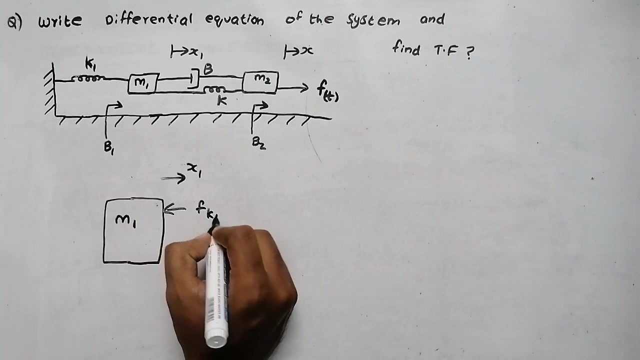 Now check whether there is any displacement Across m1. we can see a displacement x1.. So we are going to draw x1.. We need to check how many opposing forces are there. See, there is a spring. So, due to this spring, there will be an opposing force, Opposing force. this is the k1.. So I am writing fk1.. Due to 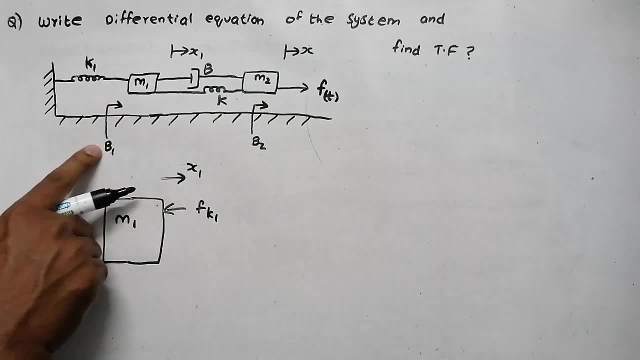 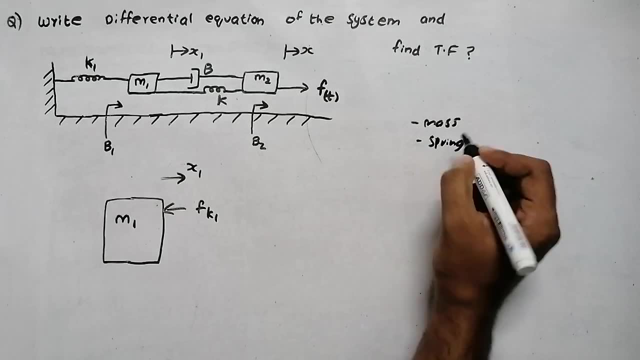 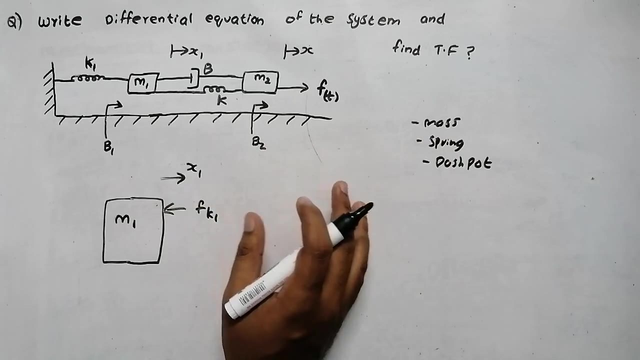 this spring there will be opposing force. Then this b1.. b1 is a damping coefficient due to dashboard. What are the three elements? Mass, spring and dashboard. These are the three elements to model a or to model a mechanical translational system. So spring is there Due to the spring. 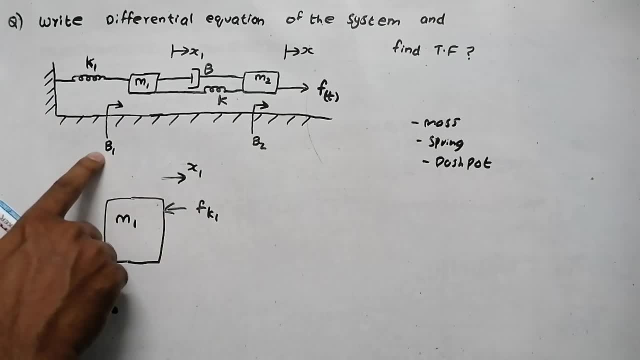 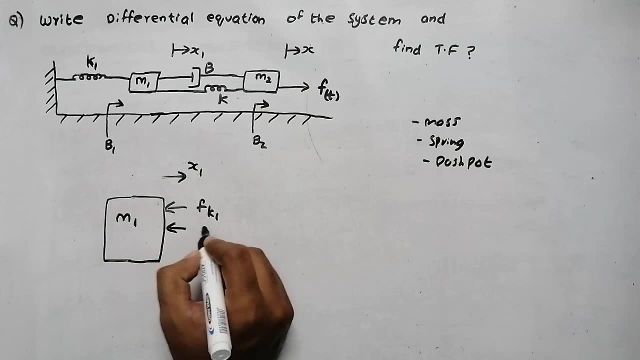 there will be opposing force, I am denoting with fk1.. Then this is a dashboard: Dashboard. the coefficient is b1.. So, due to dashboard, there is an opposing force. I am going to denote it as fb1.. Then, due to this spring, there will be an opposing force that is fk. Then, due to this, 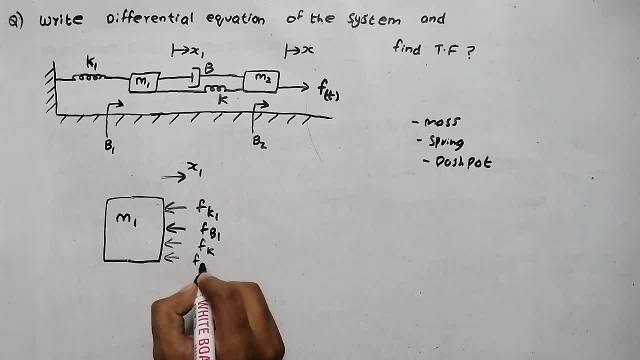 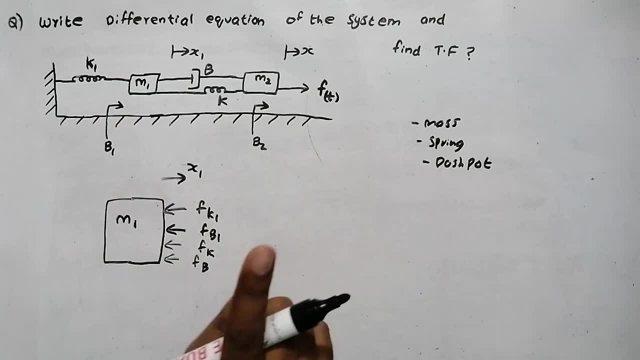 dashboard. there will be an opposing force- I am going to denote it as fb Now over: 1,, 2,, 3, 4.. Over, not over. There is one more opposing force that is due to our mass, So we will write fm. So this many opposing forces are there: 1,, 2,, 3,, 4 and 5.. 5 opposing. 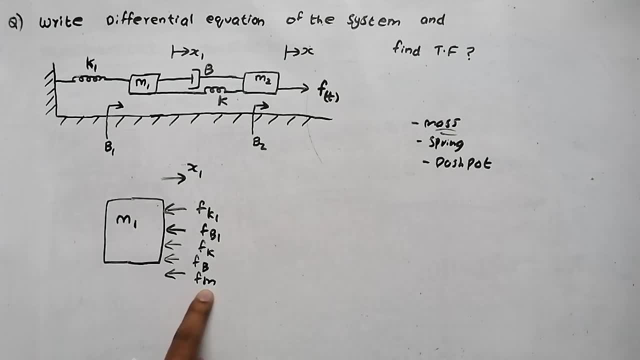 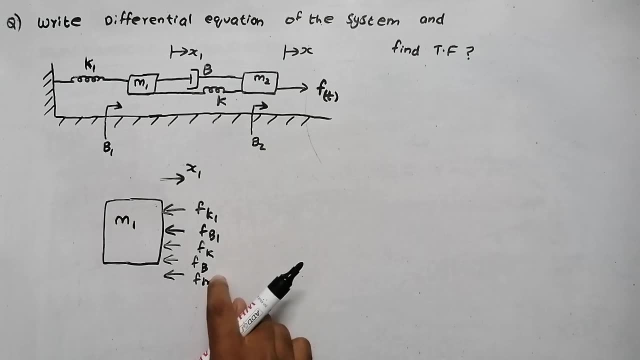 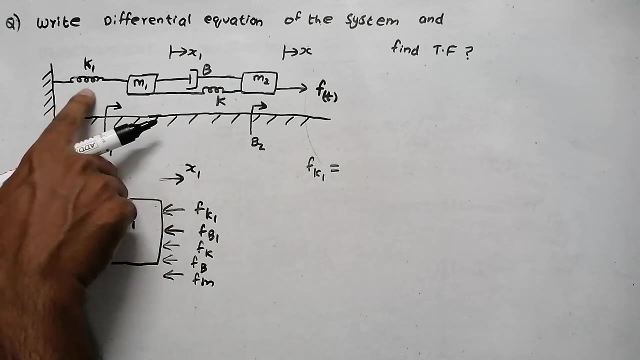 forces are there. Don't forget to write this: opposing force due to mass. So this is the free body diagram of mass m1.. Now we need to find these forces individually. So first of all we can find fk1.. fk1. It is due to spring k1. So due to spring the fk, it is What? 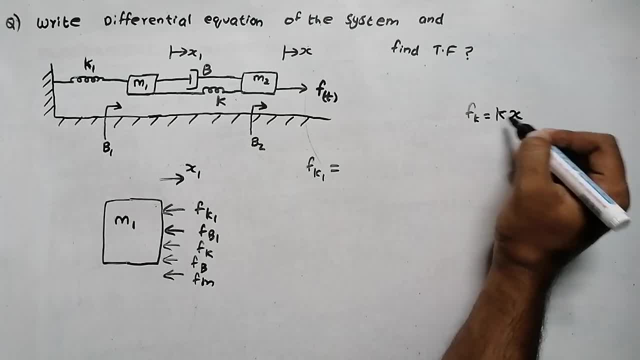 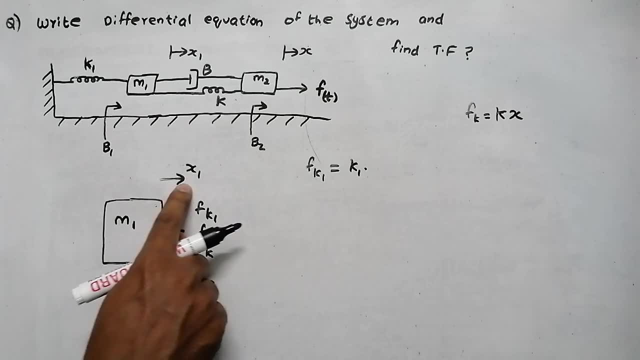 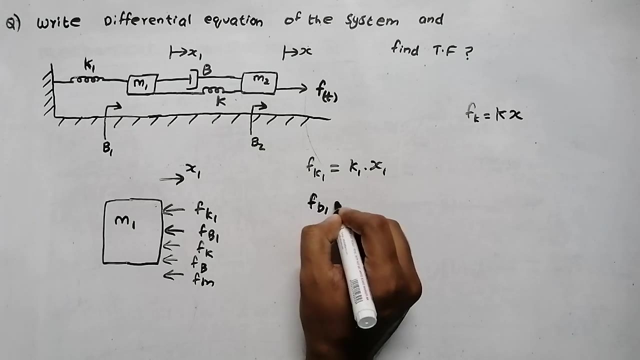 is the force equation: k into x, K is the stiffness and x is the displacement. So here, k it is k1.. So k1 into x, it is x1.. So k1 into x1.. That is our fk1.. Now fb1.. fb1 is equal to What is the? 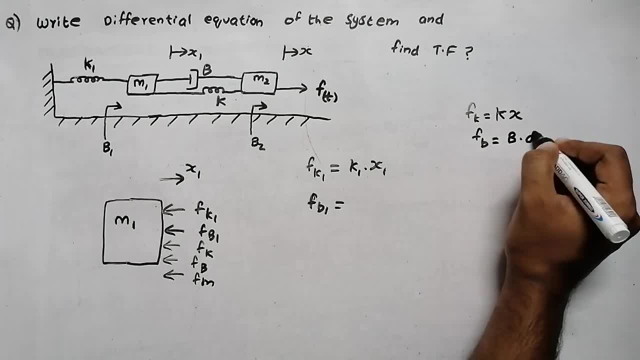 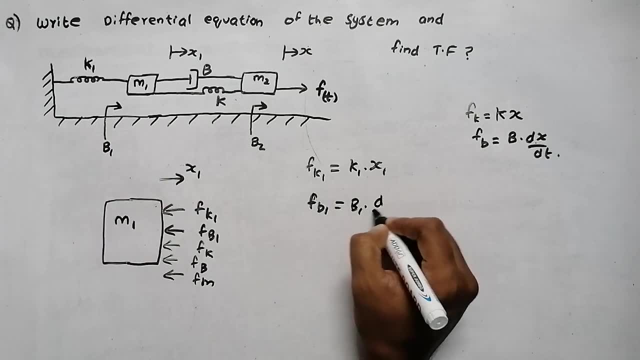 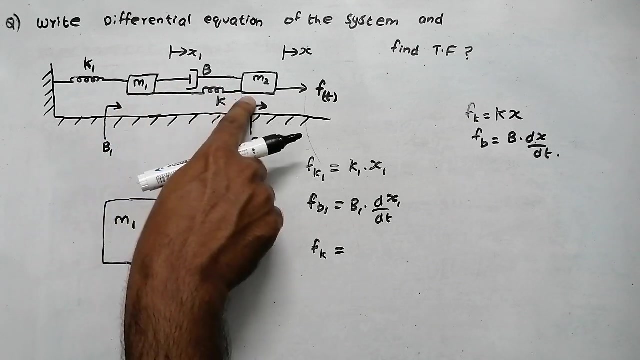 force. due to dashboard, it is b, dx by dt, so here it is b1, so b1 into d by dt of x1. due to mass m1, it is x1, now fk, fk, so k is a spring. this spring is connected to both mass 1 and mass 2. it is not. 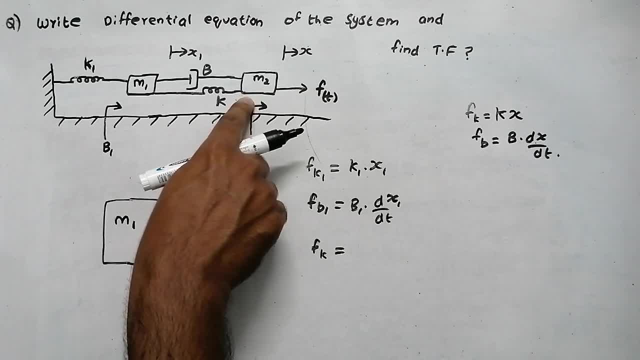 connected to a rigid body. it is connected to both mass 1 and mass 2. so for spring it is k into x, so we will write k. here it is k, so here it is k. but this k, this spring is common to both mass 1. 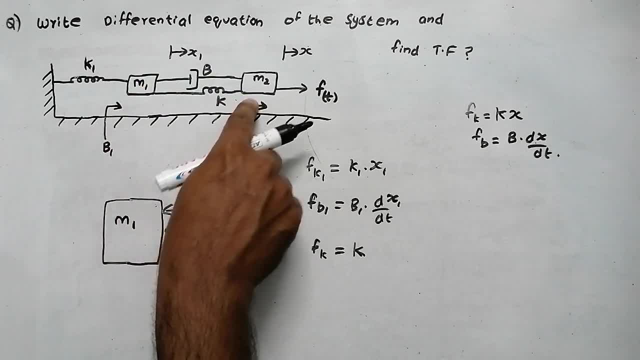 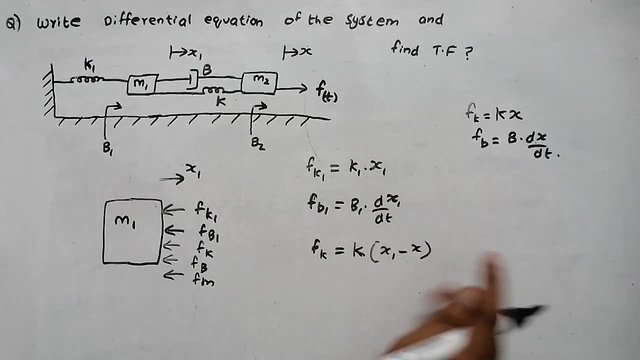 and mass 2. for mass 1, displacement is x1. for mass 2, the displacement is x. so we will write. we will write x1 minus x. why we write x1 minus x? now we are drawing free body diagram of mass 1. mass 1, so k. 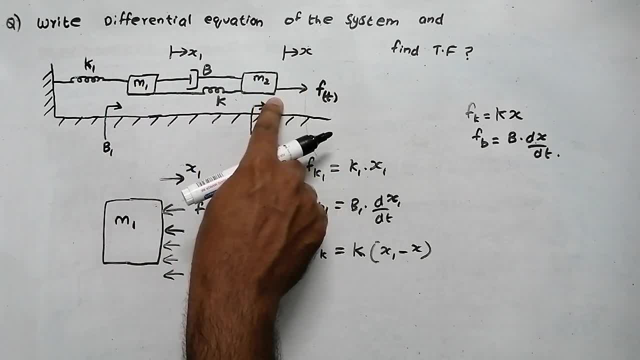 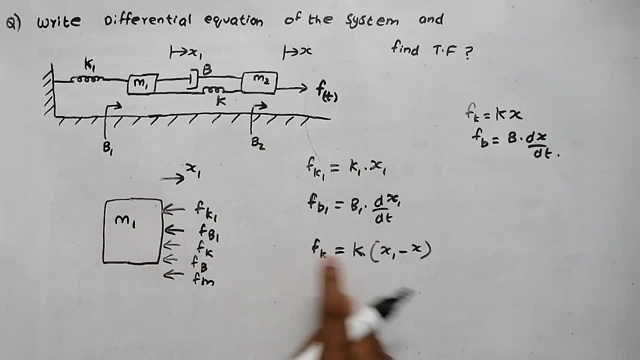 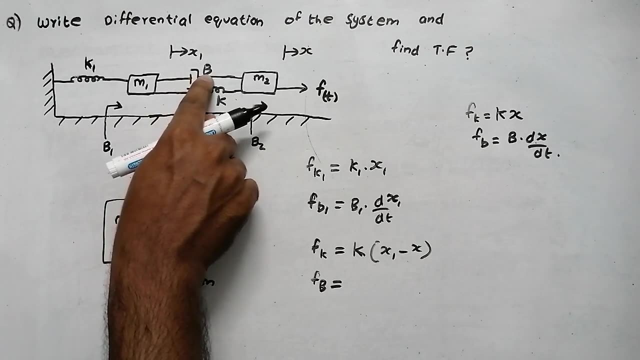 into x1 minus x. if you are writing with respect to m2, we will write x minus x1. okay, so here we are going. free body diagram with respect to mass m1. so we wrote x1 minus x. so fk is over now. fb. fb, it is dashboard. see, this dashboard is common to both masses m1 and m2. for dashboard: the equation. 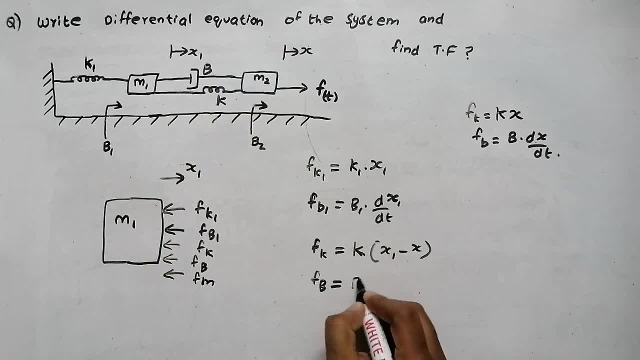 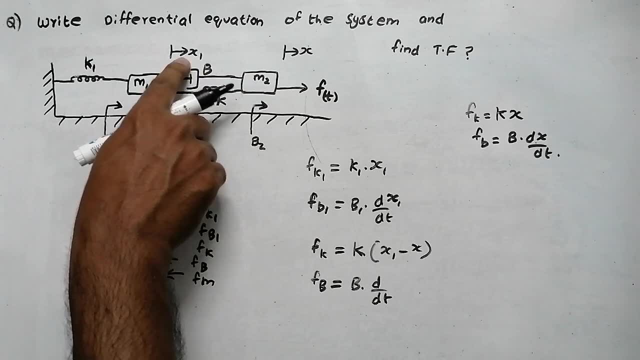 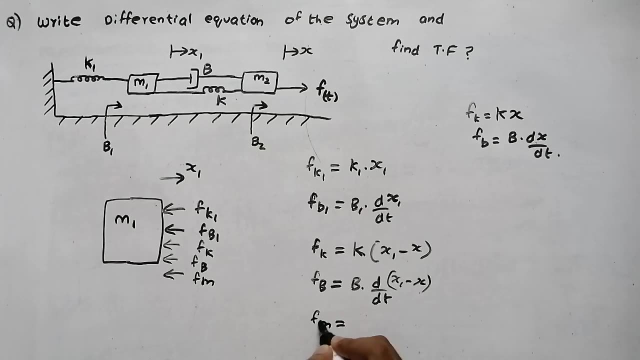 is b into dx by dt. so here it is b, so b, now d by dt of see 2. it is common to mass 1 and mass 2, so we will write x1 minus x, x1 minus x. now the last one, fm force due to opposing force, due to mass. so for mass, the opposing force, it is mass into acceleration. 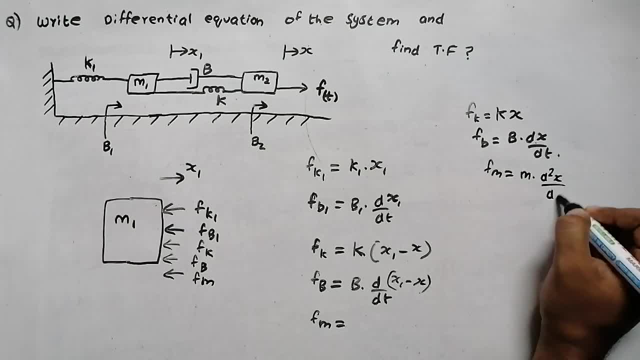 mass into acceleration means d square x by dt square. so we will write m m1. we are drawing with respect to mass 1, so m1 into d by d square, by dt square of x1 minus x2. so we will write x1 minus x1. 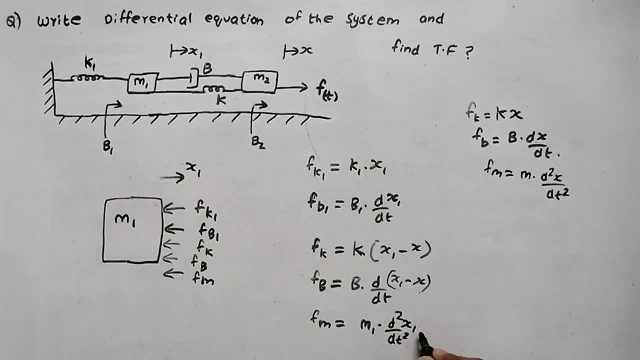 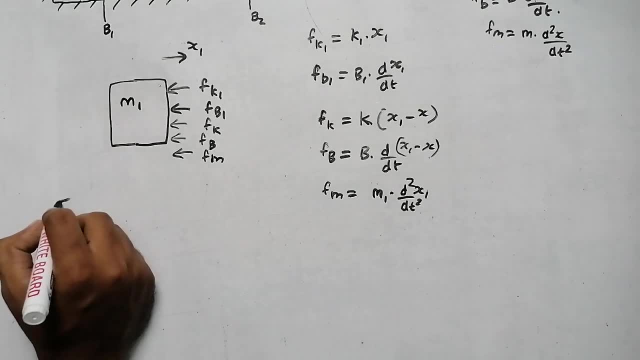 1 with respect to mass 1, the displacement is x: 1. so you write like this: m 1 into d square, x 1 by dt square. now, according to newton's second law, we know the sum of forces will be equal to 0. 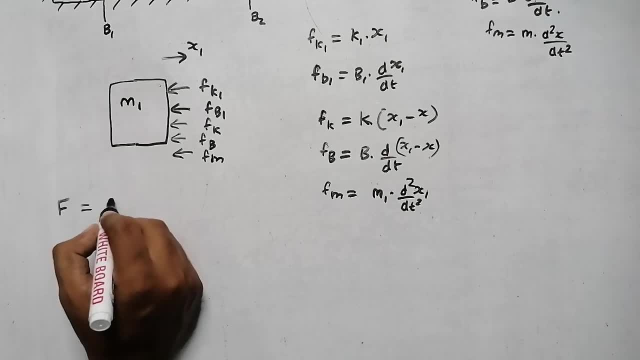 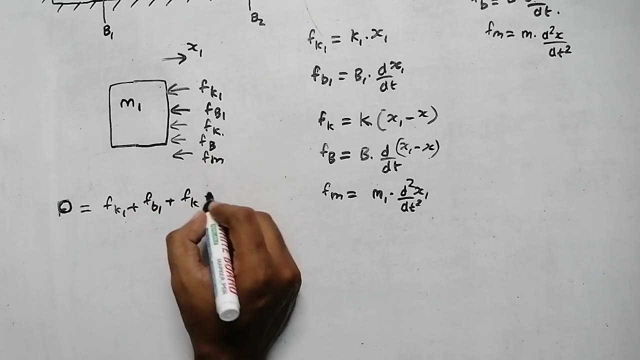 so applied force is capital f and opposing forces: are this many forces here? there is no applied force, so we will write 0. okay for m 1, there is no applied force. now. the opposing forces are fk 1 plus fb 1 plus fk plus fb plus fm. so sum of all those opposing force will be equal to 0. 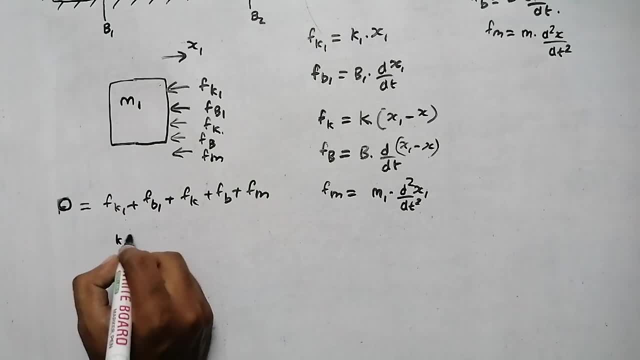 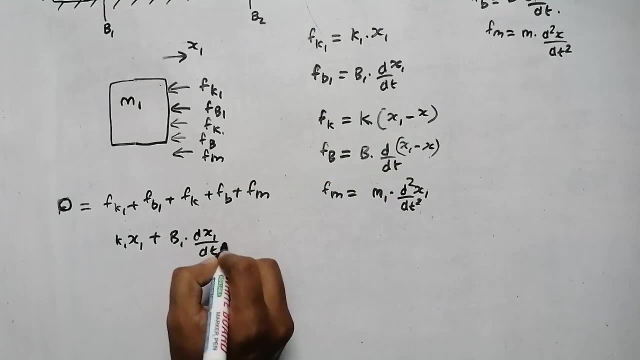 now fk 1, fk 1, it is k 1 into x 1 plus fb 1, fb 1, it is b 1, dx 1 by dt plus fk. fk, it is k into x 1 minus x fb, fb, it is b into. 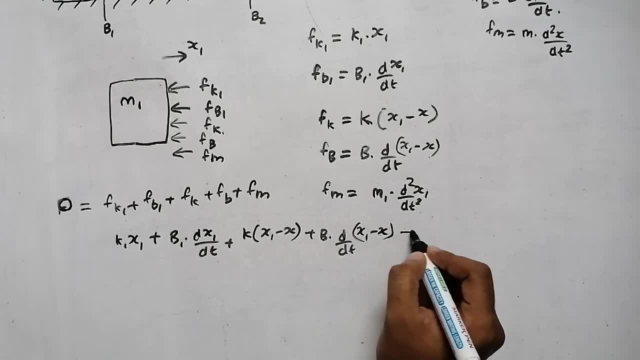 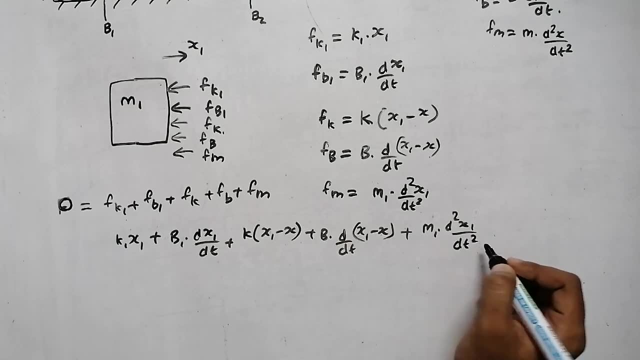 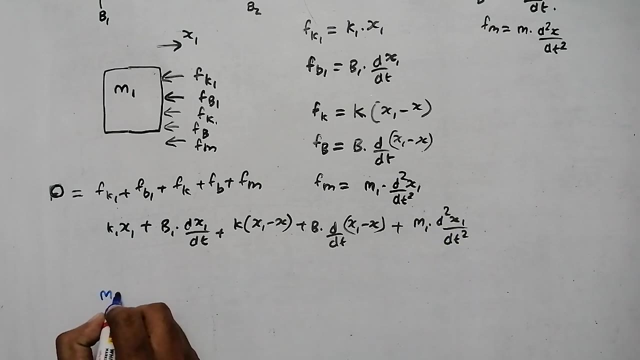 d by dt of x1 minus x plus fm, fm, it is m1 into d square, x1 by dt square. Now we can write this in a proper order. First of all, we can write the d square term, that is m d square, x1 by dt square. 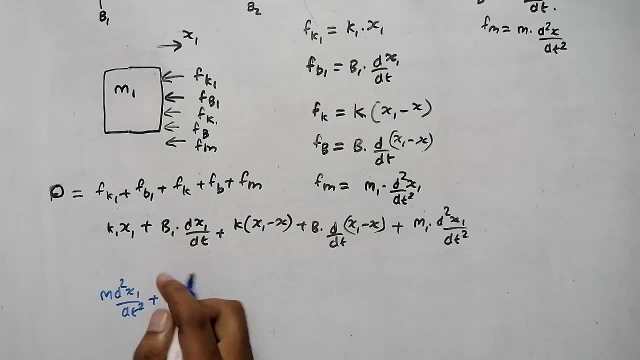 plus. then we can write the dx by dt times. So first of all we can write this term b1 into dx1 by dt plus b into d, by dt of x1 minus x plus the remaining times, that is k1, x1 and this one. 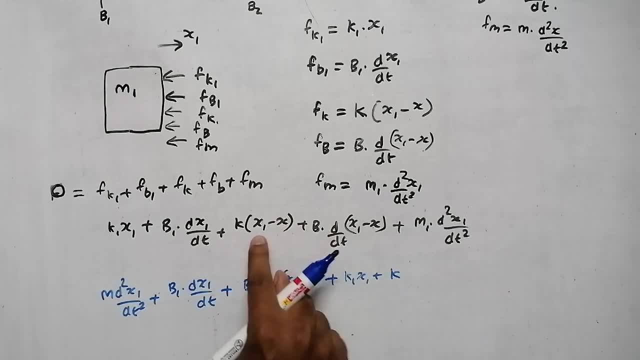 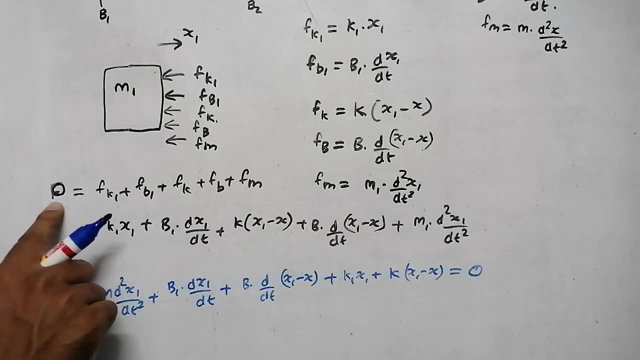 So k1, x1 plus k into x1 minus x, x1 minus x, which is equal to zero. according to Newton's second law, the sum of forces will be equal to zero. Here there is zero because there are no applied force. Now this is a differential equation: dx by dt. 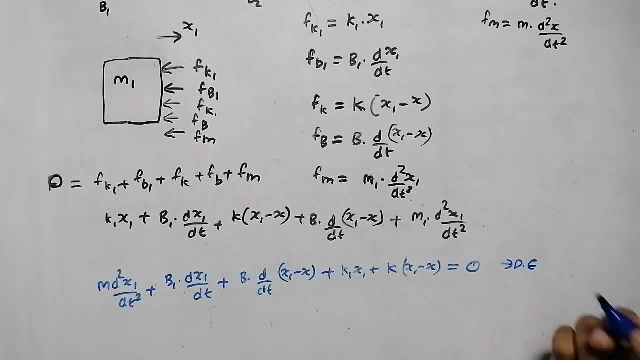 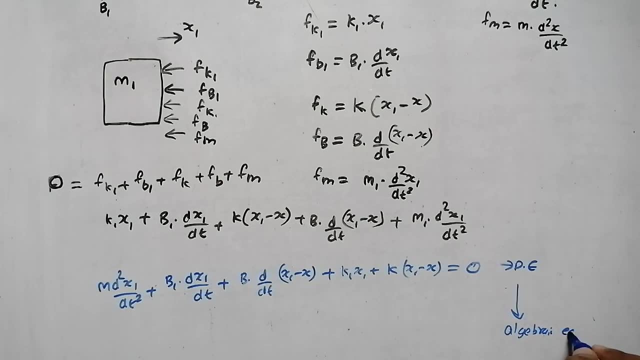 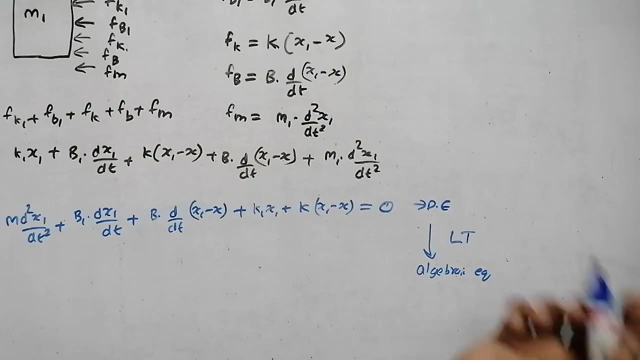 See, this is a differential equation. Solving differential equation is not so easy, So we will convert differential equation into algebraic equation. How we will convert: We will convert differential equation to algebraic equation using Laplace transform. So Laplace transform of d by: 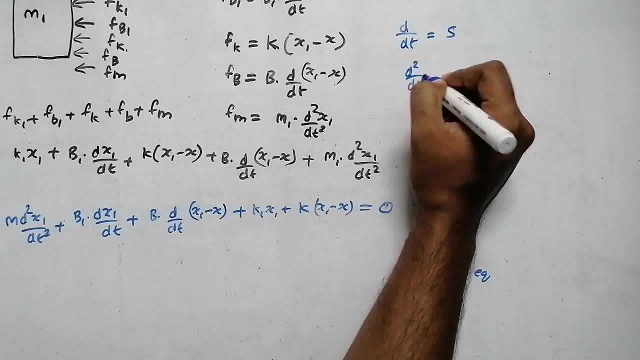 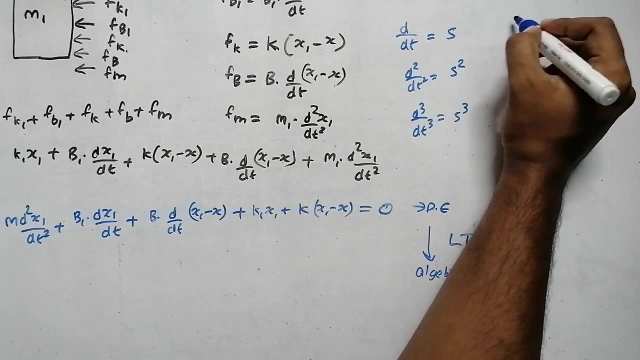 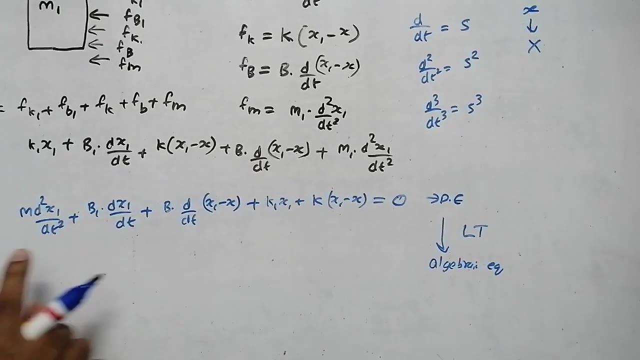 dt, it is s d square. by dt square, it is s square d cube. by dt cube, it is s cube. Now, if smaller is smaller tricks x will be converted into capital X. Okay, so here there is mass m. mass m is. 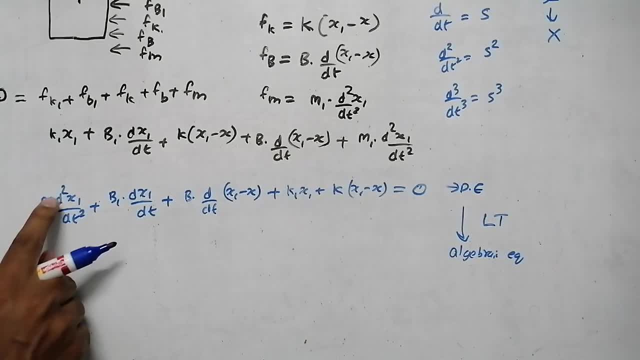 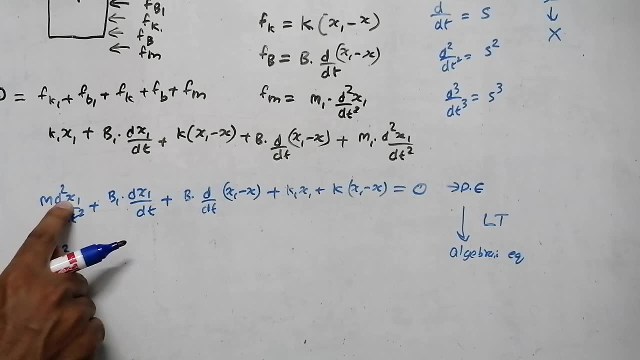 a constant, so we will write like that. Then d square by dt square, d square by dt square, it is s square, So we will write s square. then small X one. it will be converted into capital letter x. So capital x1 of x1 of s. Okay, due to the laplace transform, you write x1 will be d by dt square. it will be converted into capital X. 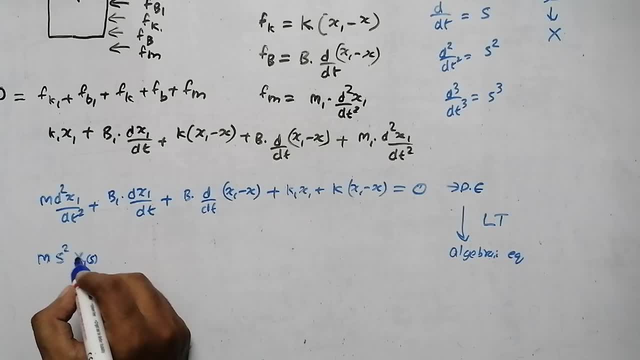 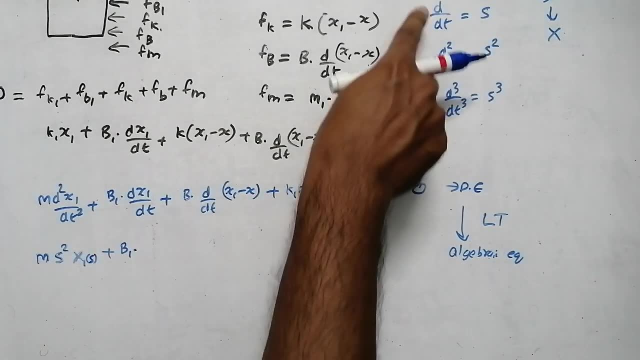 So capital X computations be 0. So capital M is less than or equal to 0, is equal to z. There are Milli of s plus b1. b1 is a constant. we will write like that itself. then. b by dt, b by dt, we will write s. 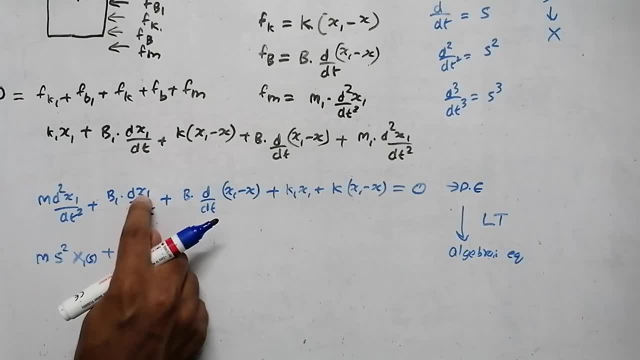 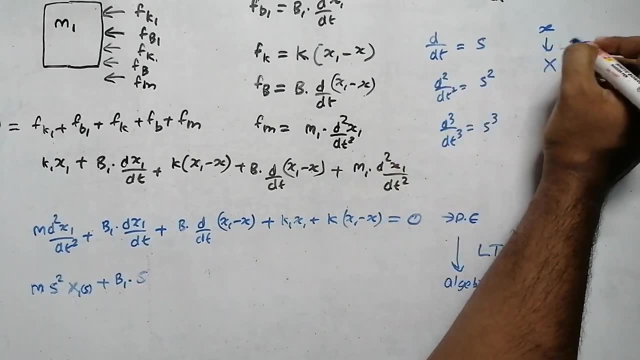 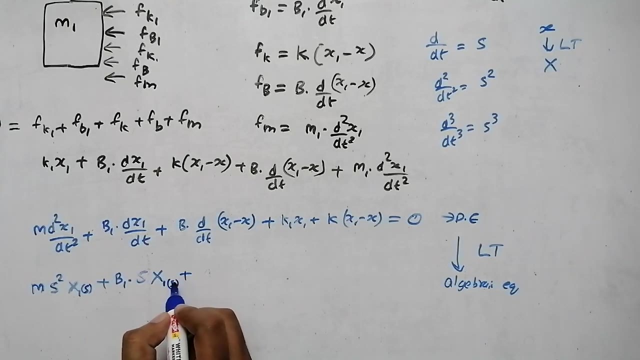 s, then x1, x1. small letter x will be converted into capital letter x. small letter x will be converted into capital letter x in laplace transform. so small letter x1 will be converted into capital letter x1 of s, because it is laplace. transform now b: b is a constant. d by dt, d by dt. 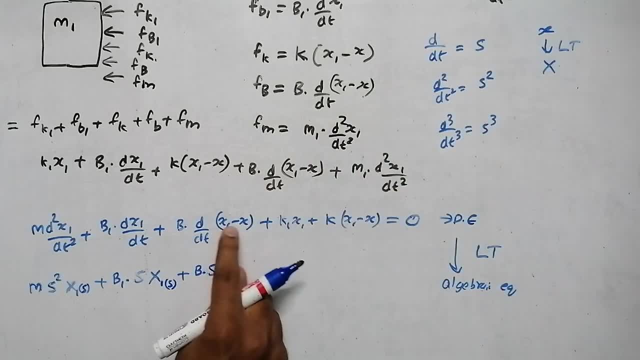 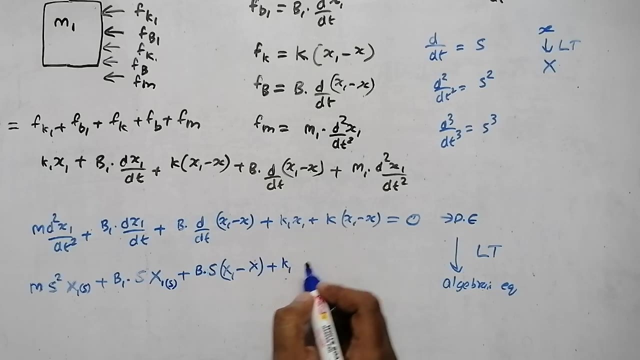 it is laplace transform, we will write s. then x1 minus x- small letter x will be converted into capital letter x. so x1 means capital x1 minus small letter x plus k1. k1 is a constant. we will write like that. then x1- small letter x1- will be converted into capital letter x1. 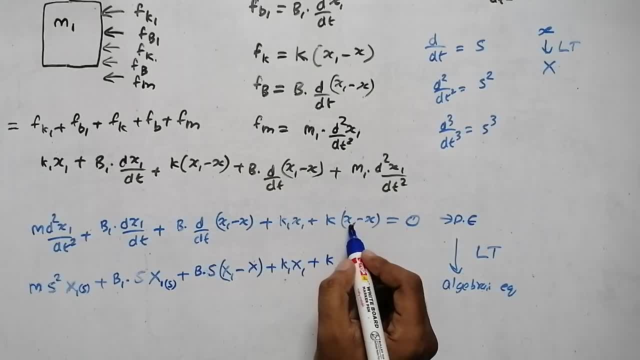 x1, x1, x1 plus k is a constant. we will write like that then: small letter x, 1 will be converted into capital letter x 1 x 1 of s, is there? okay? minus x will be smaller. tricks will be converted into capital x. we will write this smaller x of s later, okay, or you will have a confusion. 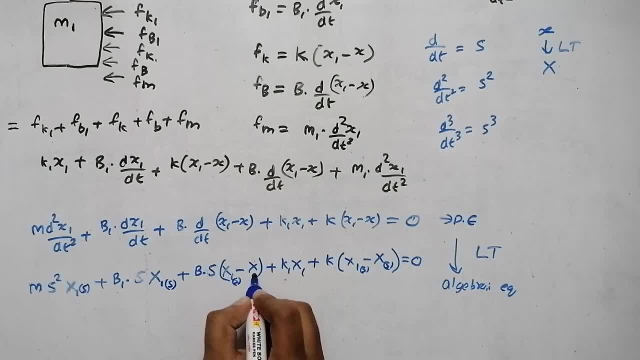 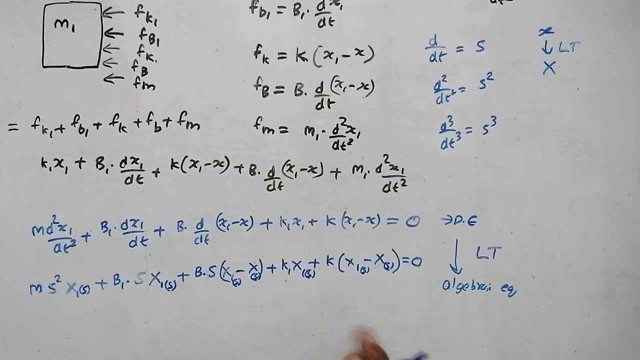 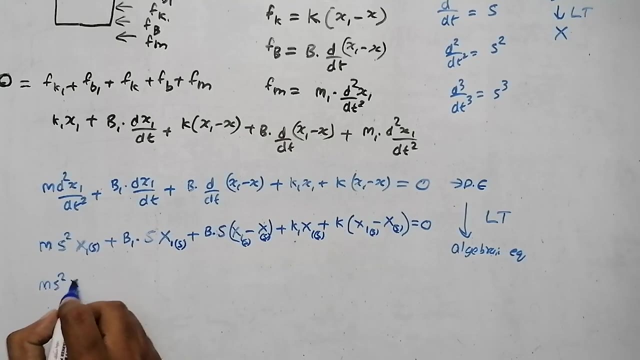 since we are converting into laplace transform, we need to put a suffix x, x of s, like that: for all x. we need to put that bracket in bracket. you need to put this s now open all the brackets here. there are no brackets, so you write like that itself: m square x 1 of s plus b, 1 s x 1 of s plus here. 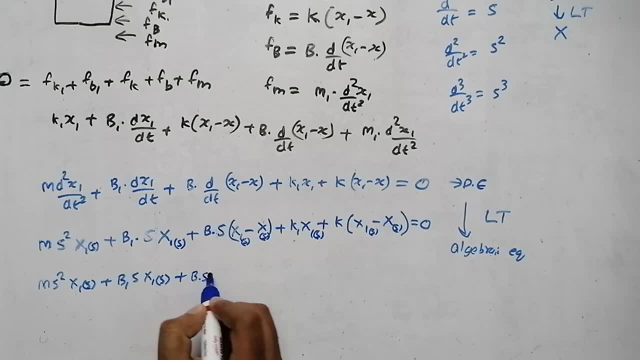 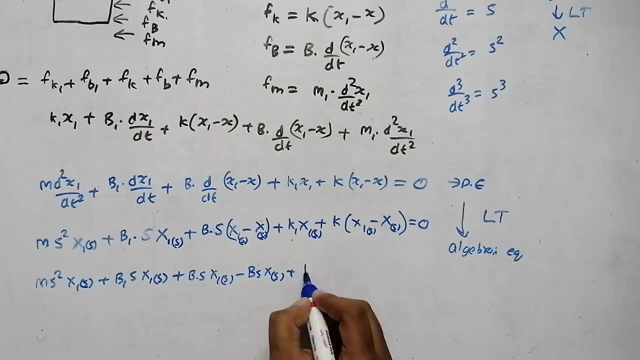 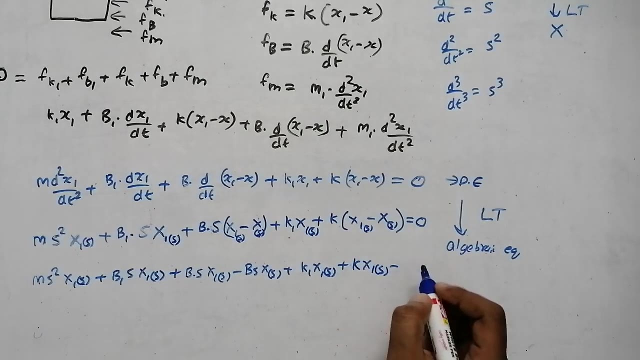 there is bracket, so open this bracket. it will become b s x 1 of s minus b s x of s plus k 1 x 1 of s, plus here there is bracket. open the bracket. we will get k x 1 of s minus k x of x equal to 0 now. 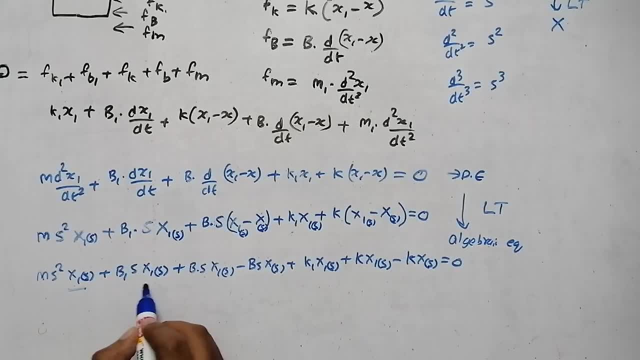 group all the x 1 times. here there is x 1, here there is x 1, here there is x 1, here it is x 1 and here it is x 1, and here it is x of s and here also it is x of s. 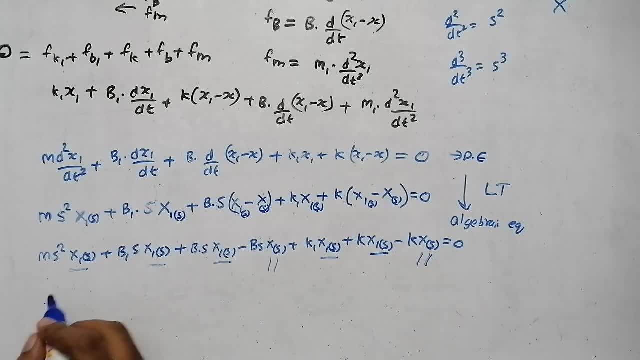 so from this, x 1 of s is common, so we are going to take x 1 of s outside. then the remaining times are m square plus b 1 s plus b s, plus this one k 1 plus k. okay, x 1 of s is common, so we took it outside. then the remaining times are m square, b 1 s, b b s, then k 1 x. 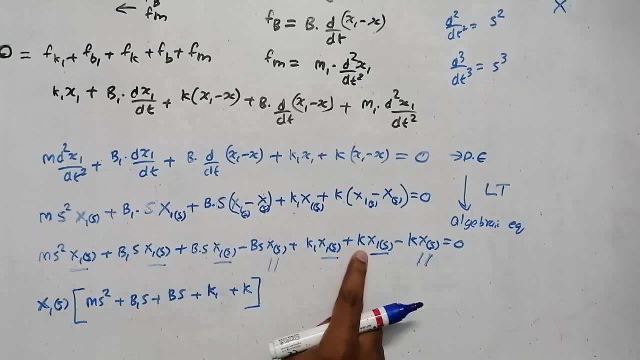 1- this time is not there because it is x of s- then k 1 and k. okay, now the remaining times are this: one minus b s, x of s, then minus k, x of s equal to 0. here x of s is common, so i'm going to take, and minus is also common, so minus x of s i am going to take outside. 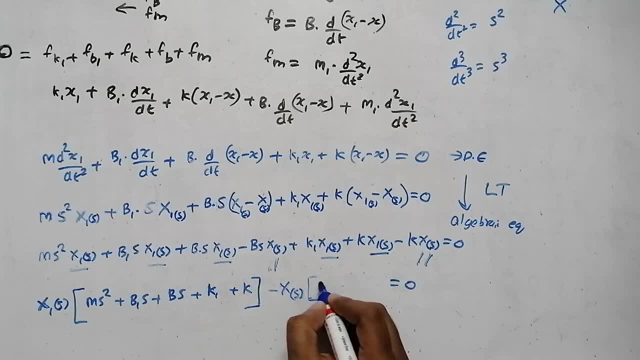 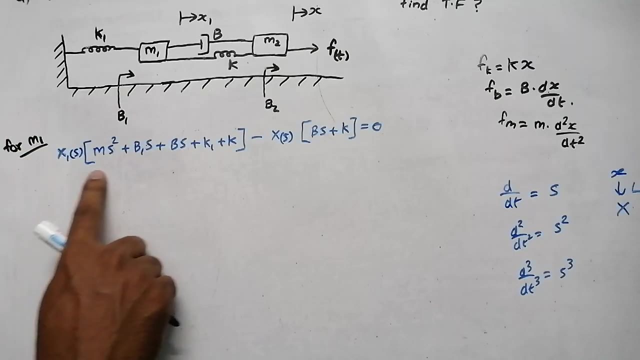 so we took minus x of s outside, then the remaining times are bes and here it is minus k. since minus is outside, we will write plus plus k equal to 0. so by taking mass 1 and drawing the free body diagram, we got the equation like this: okay, keep. 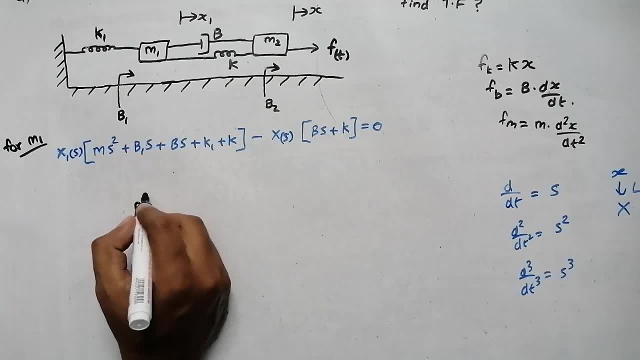 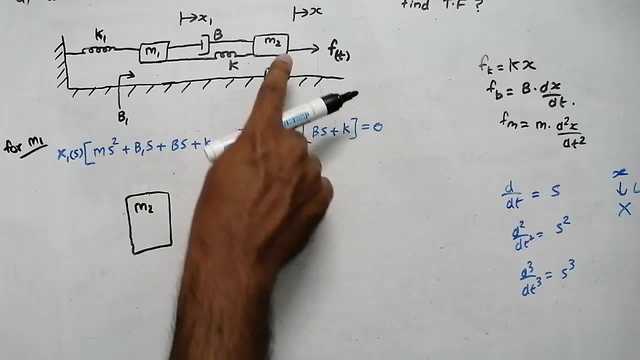 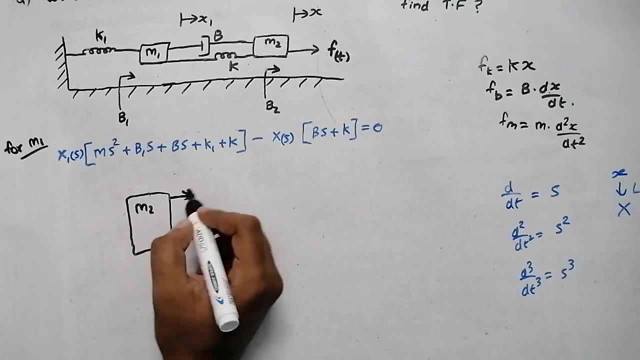 it in one side. now we are going to draw the free body diagram of mass: m 2, m 2. so first step is to check whether there is any applied force. yes, as you can see here, there is an applied force, f of t. so applied force, applied force. i am going to write in this direction: f of t. now check whether. 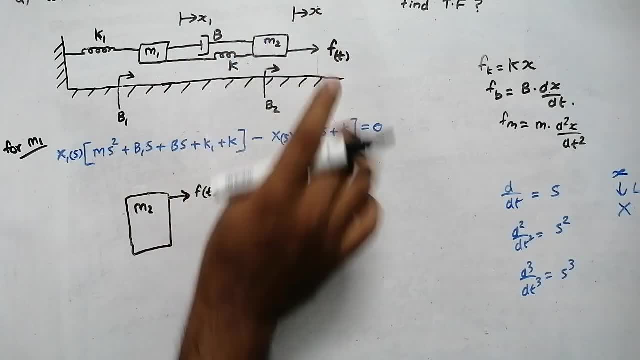 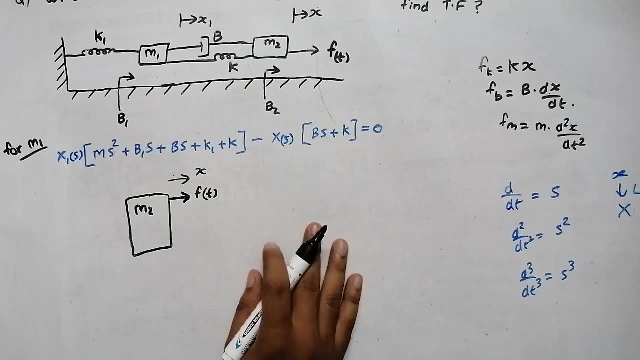 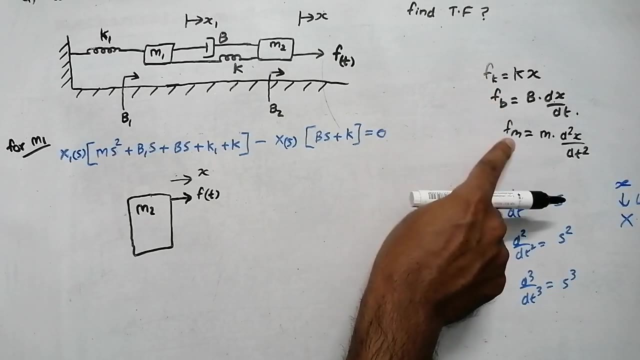 there is a displacement, applied force and displacement will be in the same direction. so there is a displacement x. now check the opposing forces. so three elements are there: mass, spring and dashboard. this is the force due to spring, dashboard and mass. so check the opposing forces. so first of all, we can see. 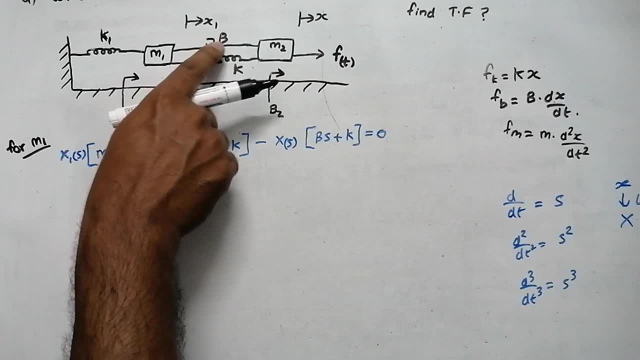 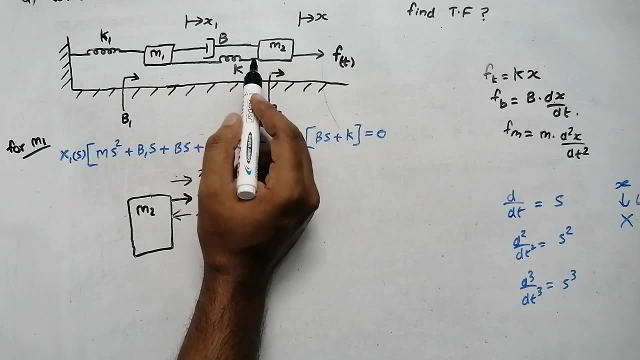 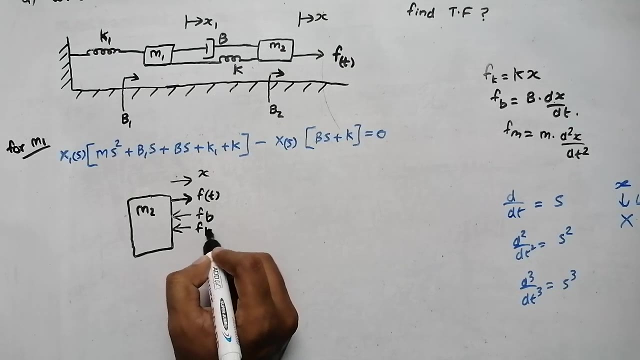 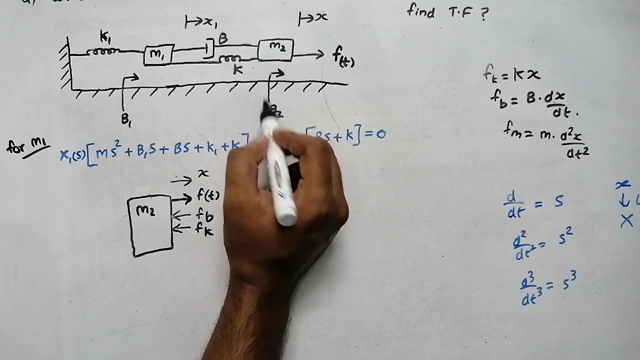 there is an b. b is for dashboard, so we will write opposing force f of b. now spring- spring is there, so we will write opposing force due to spring. that is f k, k is the stiffness constant and b is for dashboard, that is damping coefficient. now b 2. b 2 is for dashboard, so opposing force due to b 2. 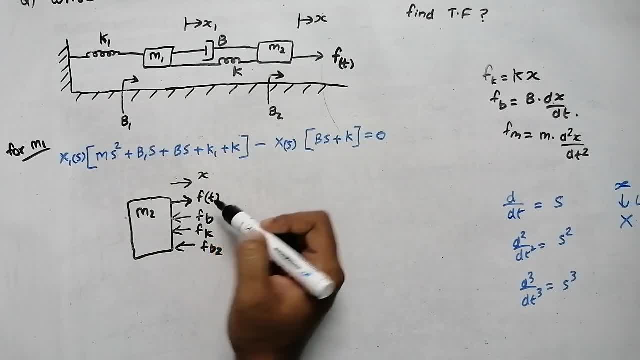 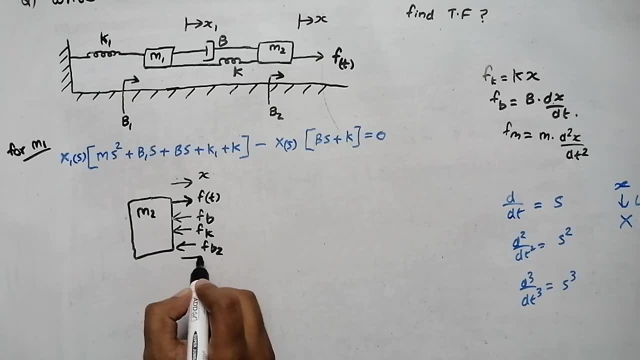 is for dashboard, that is damping coefficient. now b 2. b 2 is for dashboard, that is damping coefficient, and f? t. we already wrote so. is there any another force, opposing force? one more is there that is due to this mass. so there is one more opposing force that is due to mass m2. so one, two, three, four, four. 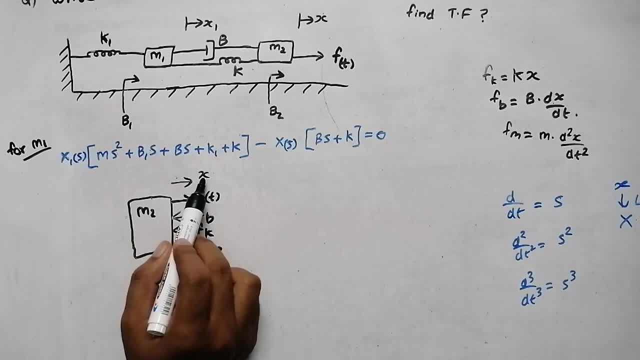 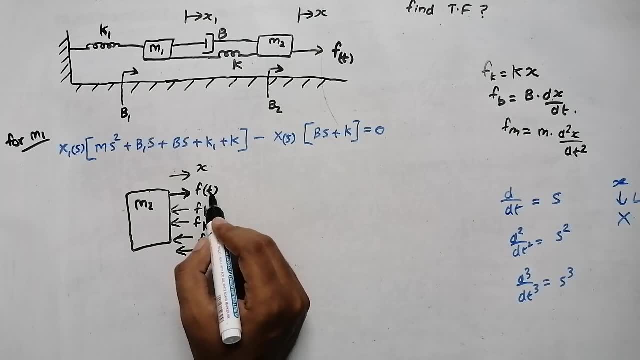 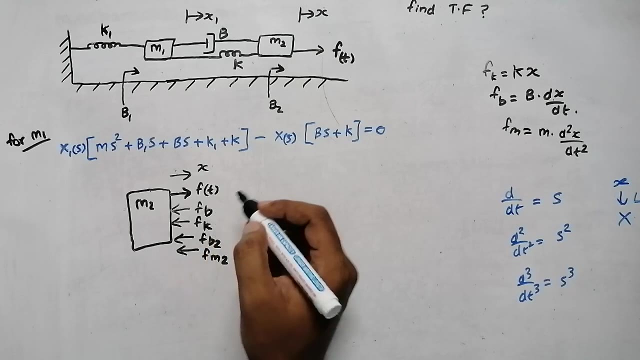 opposing forces. are there one applied force and one displacement? now we need to find these forces individually. okay, so first of all we can find f t is the applied force. let them be there. we are going to find the opposing forces. so f b, f b is the opposing force. due to this, 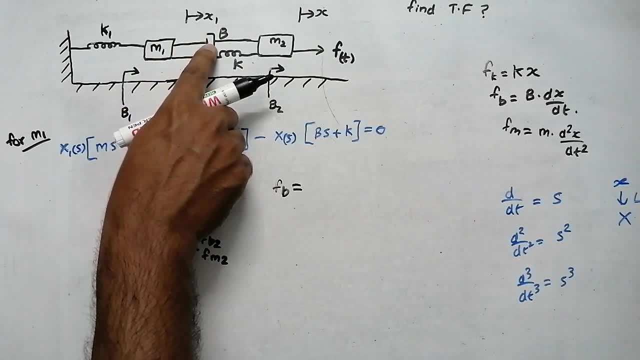 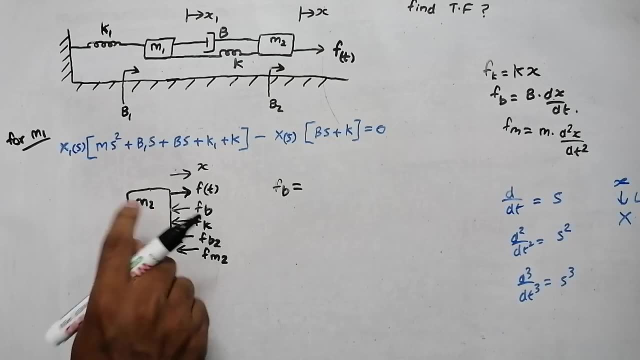 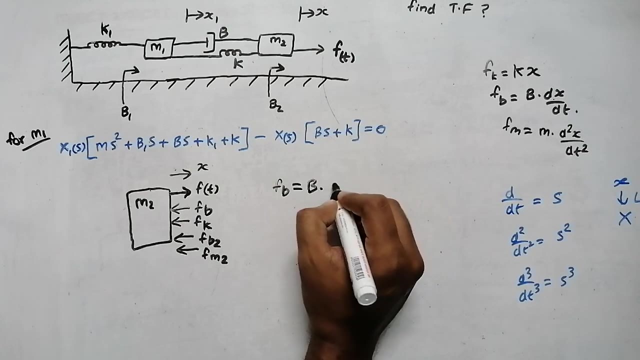 dashboard. okay, and as you can see here, this dashboard is common to both mass 1 and mass 2 and here we are drawing free body diagram with respect to mass 2. so for dashboard, the equation it is b into dx by dt, so here b, so we will write b into d by dt of. it is not dx by dt. why? because 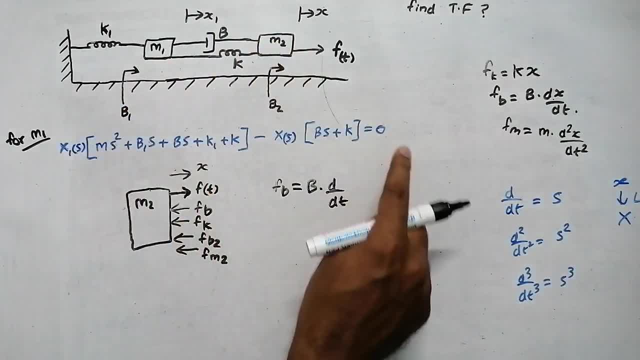 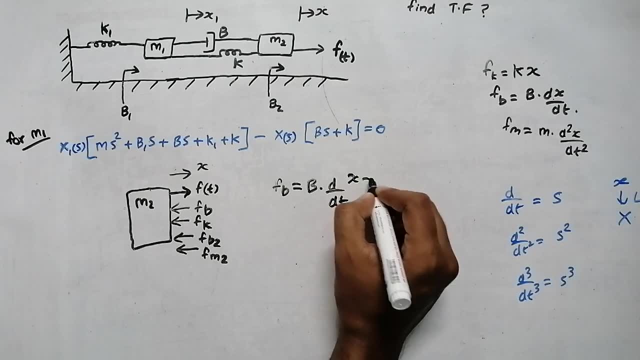 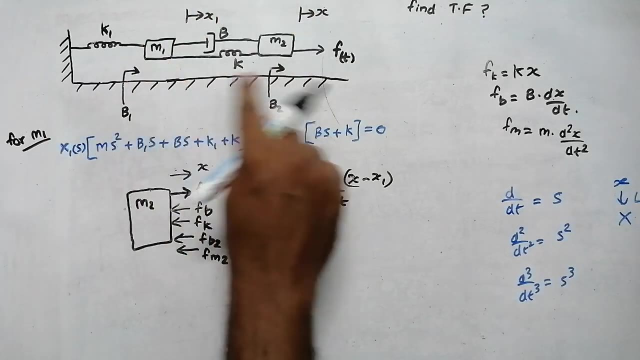 this dashboard is common to both mass 2 and mass 1.. so you will write x minus x1. x is the displacement of m2. okay, so you will write x minus x1. hope you understood. if you're writing with respect to mass 1, we will write x1 minus x. if you're writing with respect. 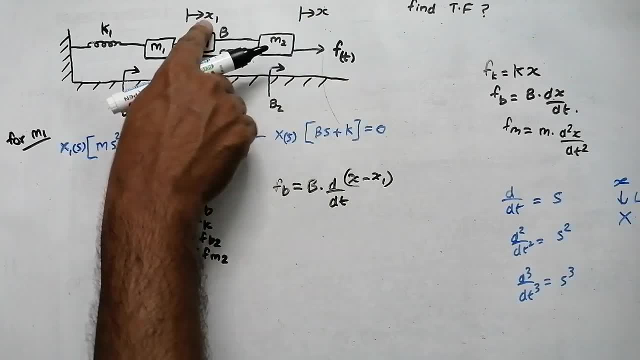 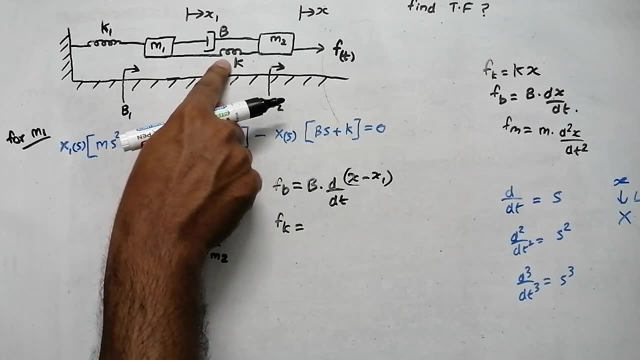 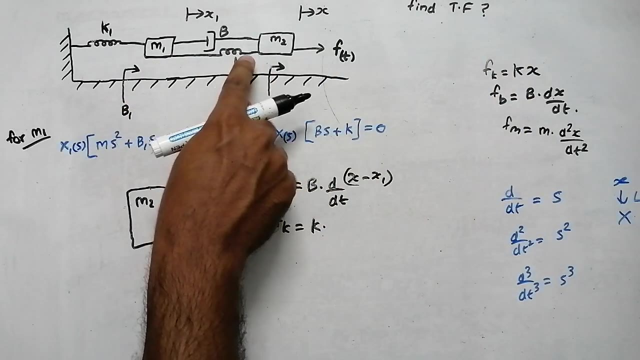 to mass 2, the displacement here. it is x, so you'll write x minus x1 now f k. f? k is the opposing force due to this spring and, as you can see, spring is common to both mass 2 and mass 1. so fk it is kx, so we'll write k then instead of x we. 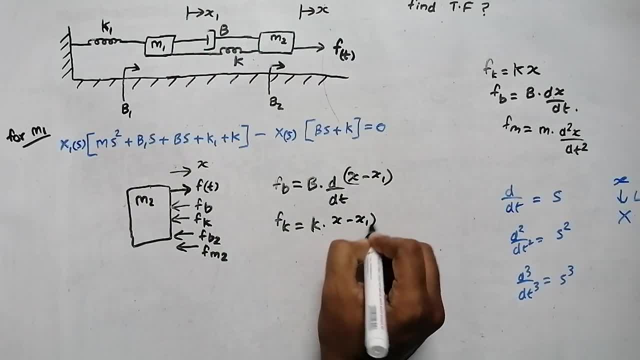 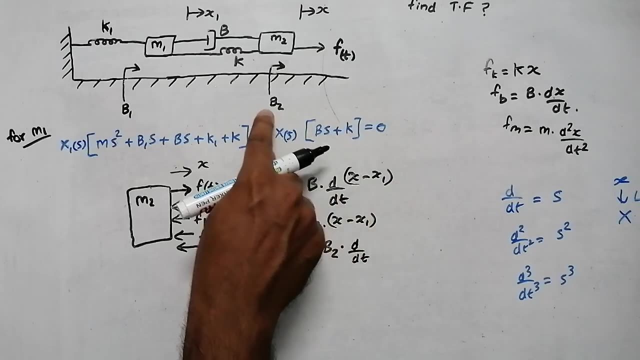 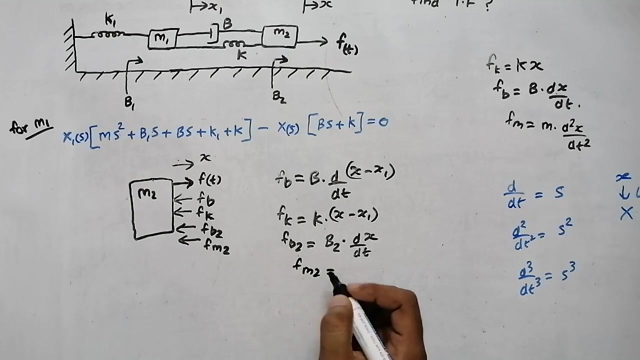 will write x minus x1, x minus x1, now fb2. fb2 is the dashboard. this dashboard coefficient. so for b2 it is instead of b. we will write b2 into d by dt of see, this is a rigid body, so there is only one displacement. that is x. now fm2. fm2 it is the opposing force. due to mass m, it will be m d square. 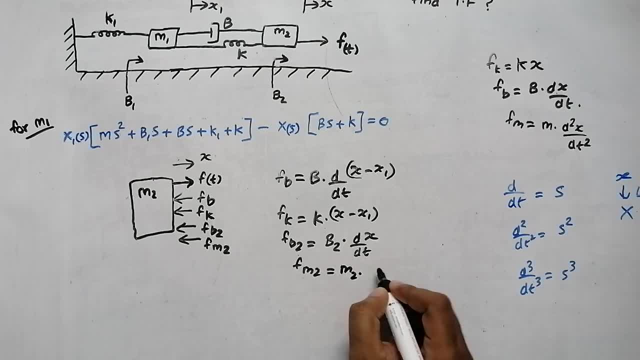 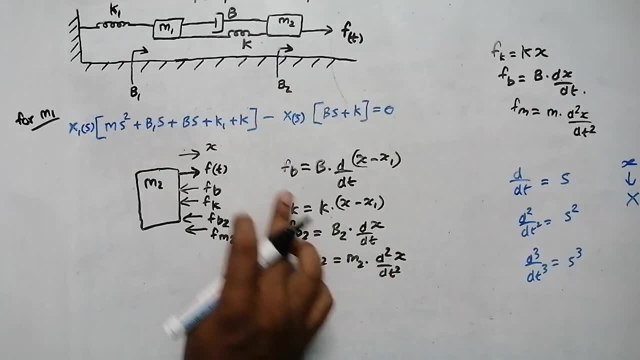 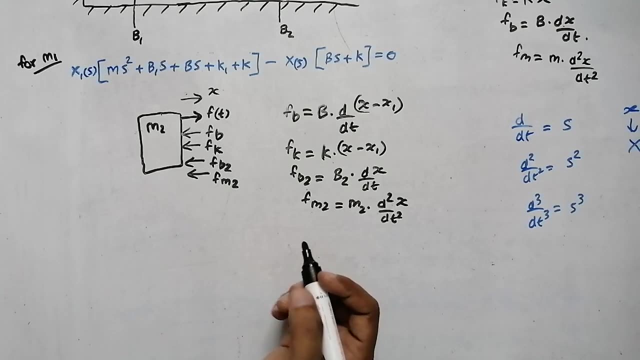 x by dt square. instead of m we will write m2. so m2 into d square by dt of dt, square of x. okay, the displacement of second body. so these are the opposing forces. now, according to newton's second law, the sum of applied force and opposing force force will be equal to zero. 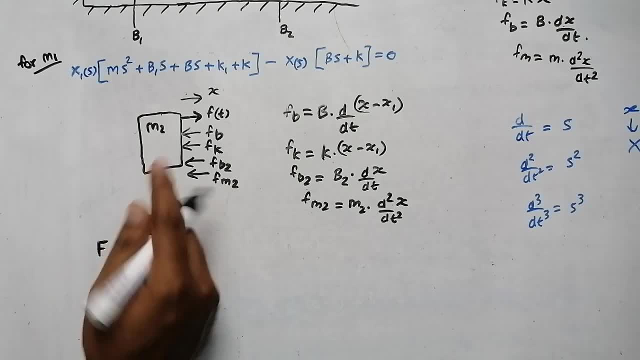 so we will write m2 into d square by dt of dt square of x. so we will write m2 into d square by dt of dt square. we will write: this is the applied force f of t. so according to newton's law, f of t will be: 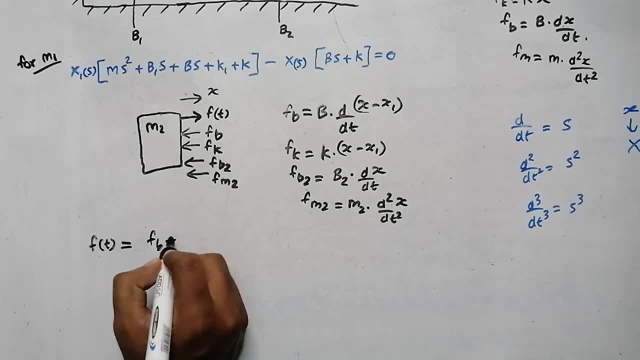 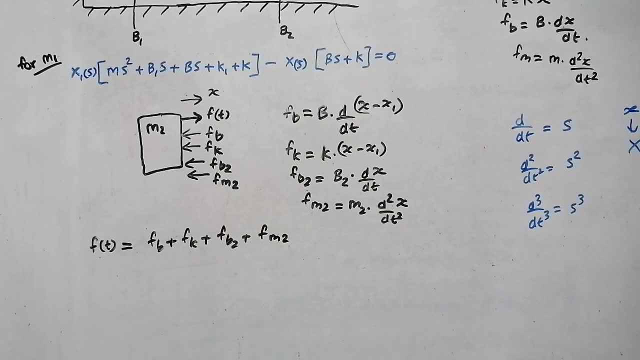 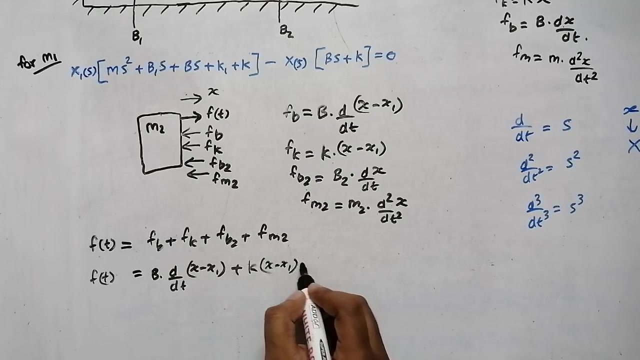 equal to the opposing forces. that is fb plus fk plus fb2 plus fm2. so fb it is b, d by dt of x1. okay, f of t. i will write like that itself then: fb, fb it is b into d by dt of x minus x1 plus f, k. f, k. it is k into x minus x1 plus f. b 2, f, b 2 it is b, 2 into dx by dt. 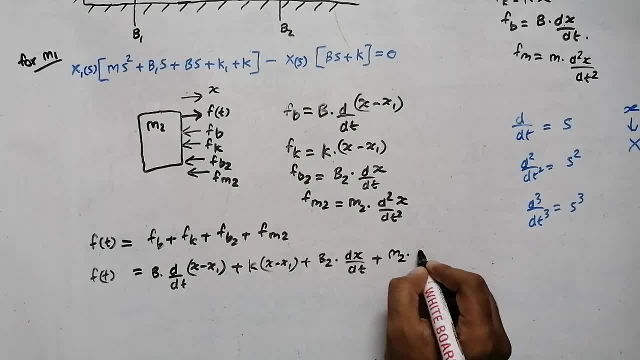 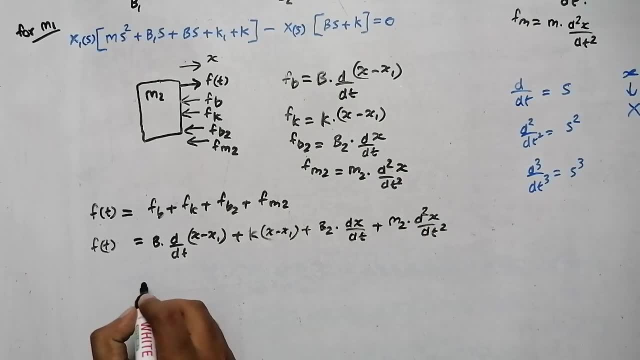 plus fm2 m2. it is m2 into d square x by dt square. now we can write this in a order. first of all write the d square type. so it is m d square x by dt square. now we can write this in a order, first of. 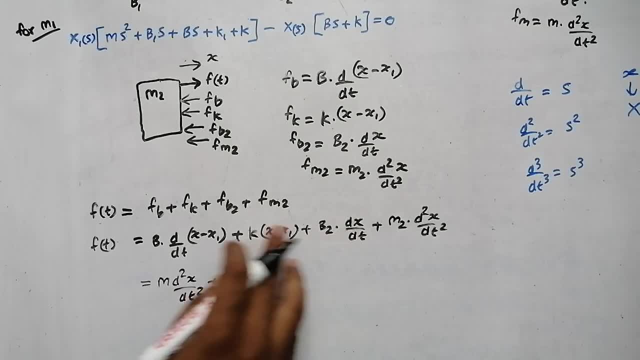 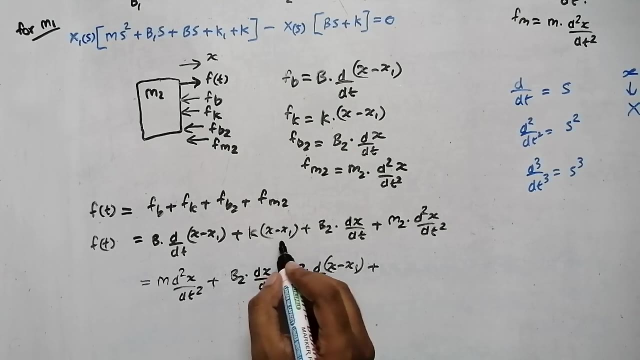 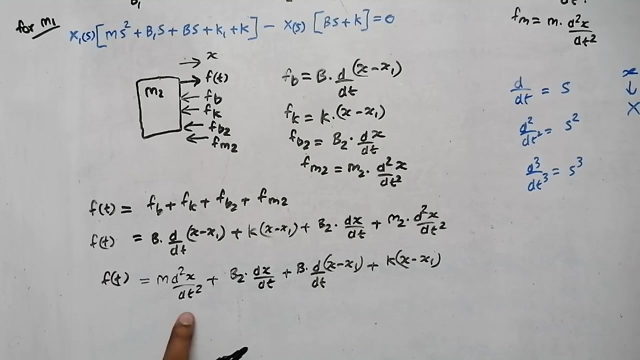 dt square, then write the d by dx, dx by dt times. so here there is one, here there is one. so first of all, you can write b2 into dx by dt plus b into d by dt of x minus x1 plus the remaining term, that is k, x minus x1, which is equal to f of t. now, as you can see here, this is a differential equation. 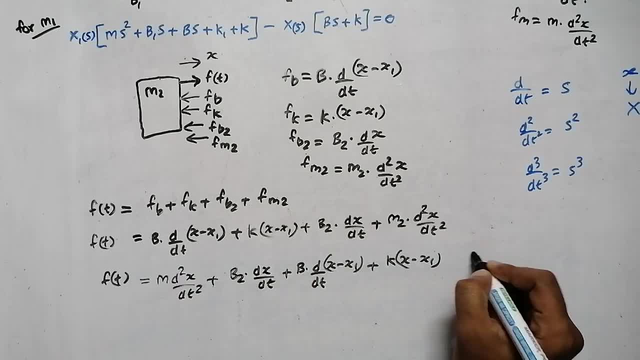 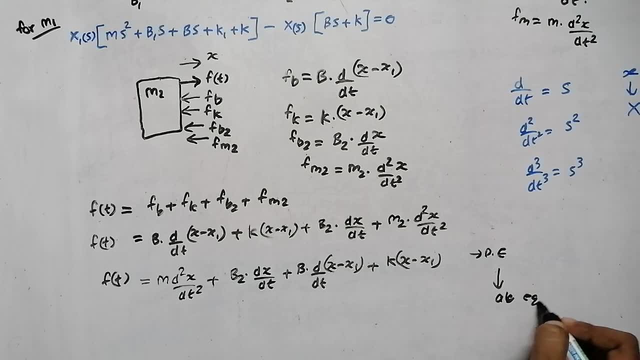 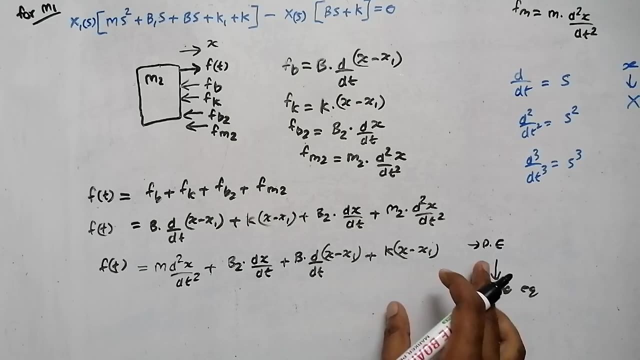 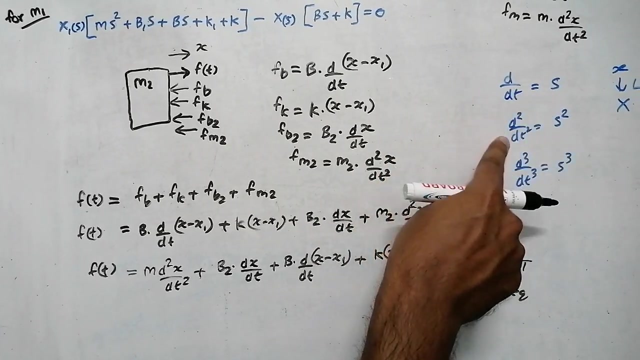 d by dt time, see dx by dt. those are differential equation. what we need to do? we need to convert differential equation into algebraic equation. why? for solving, for solving this equation, differential equation solving is not easy. so we converted differential equation into algebraic equation using Laplace transform. so d by dt, the Laplace transform, it is s d square by dt square. 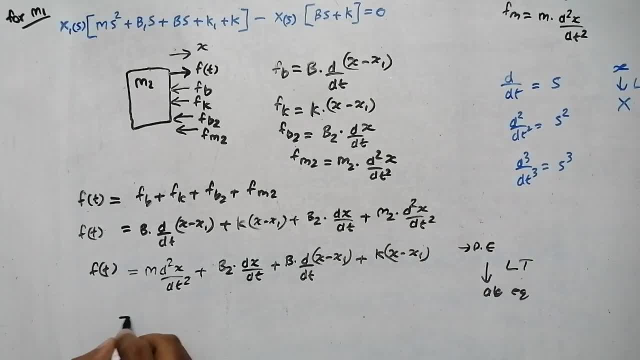 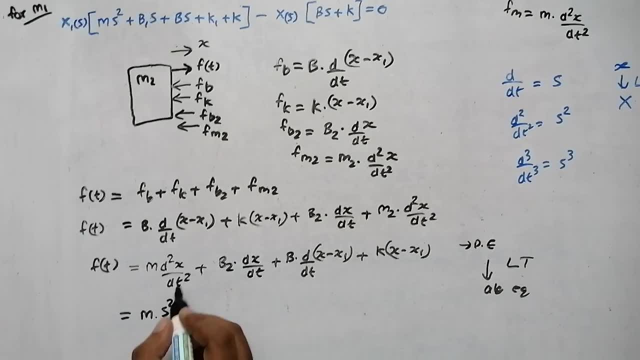 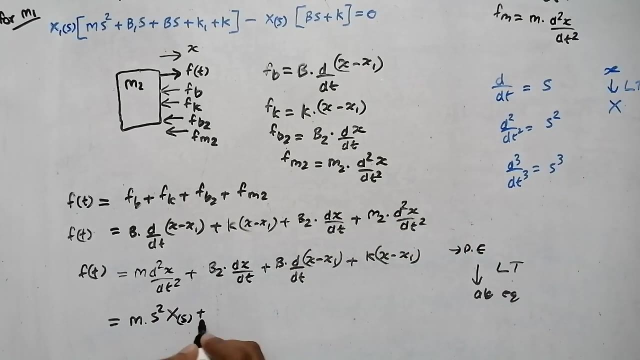 it is s square. d cube by dt cube. it is s cube. so you will write: mass is a constant. we will write like that itself and d square by dt square. that is a square. then small letter x. it will be converted into capital letter x, so it will become x of s plus then b2. 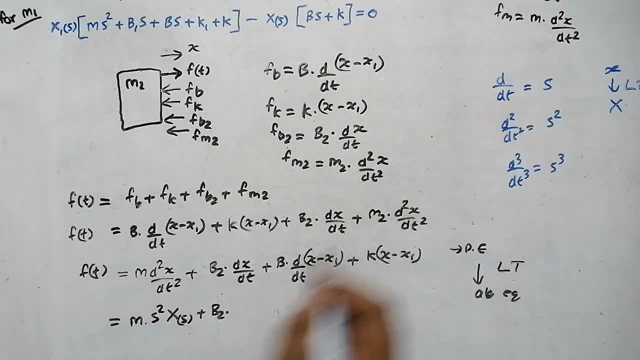 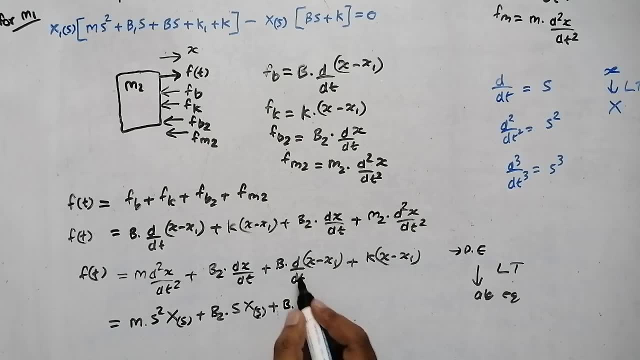 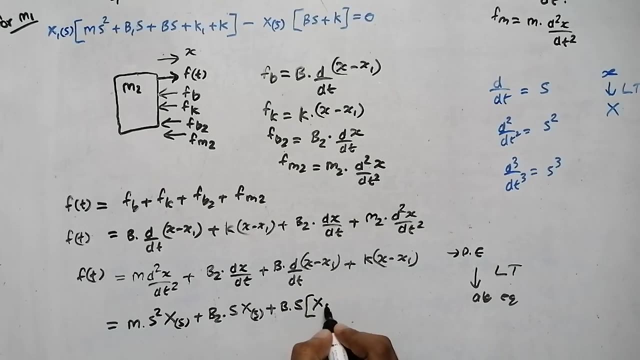 it is constant. d by dt, d by dt. we will write s. then small letter x will be converted into capital letter x of s plus b into d by dt. d by dt. we will write s. then bracket, small letter x will be converted into capital x of s minus x1. x1 will be converted into capital x of 1 x1 of s. 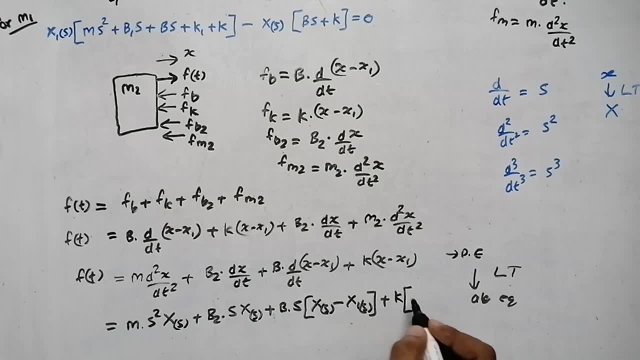 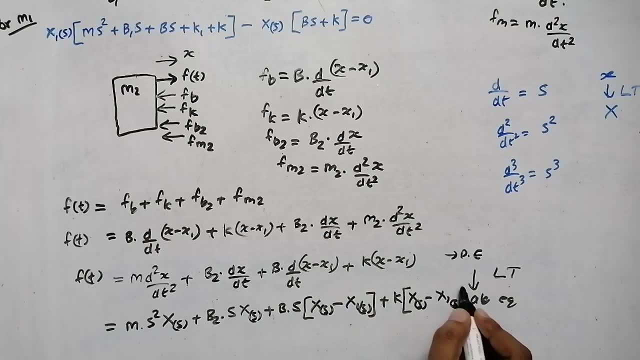 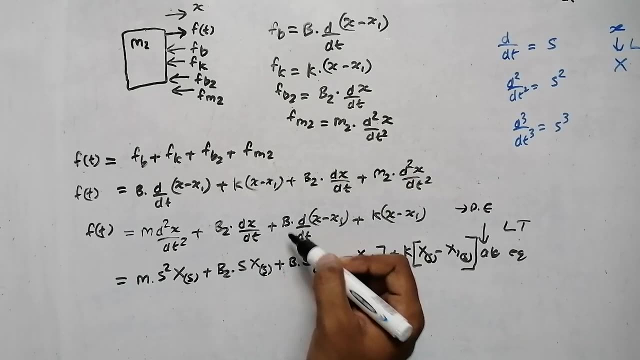 plus k in bracket, small letter x will be converted into capital x of s. minus small letter x1 will be converted into capital x1 of s. so this is the equation. now open the brackets. this is a the algebraic equation. we converted differential equation into algebraic. 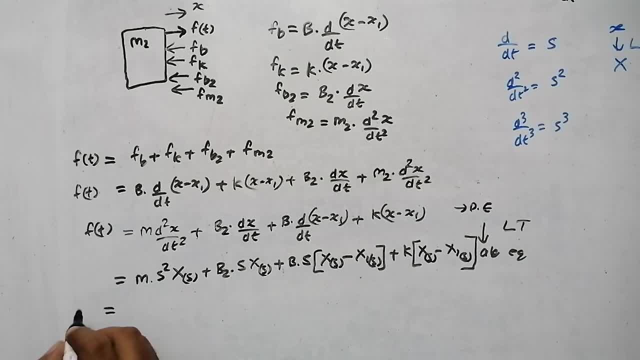 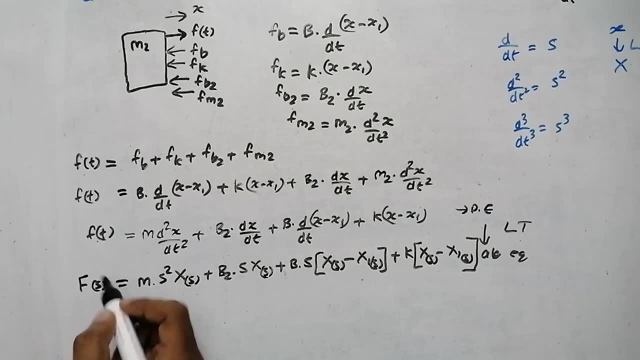 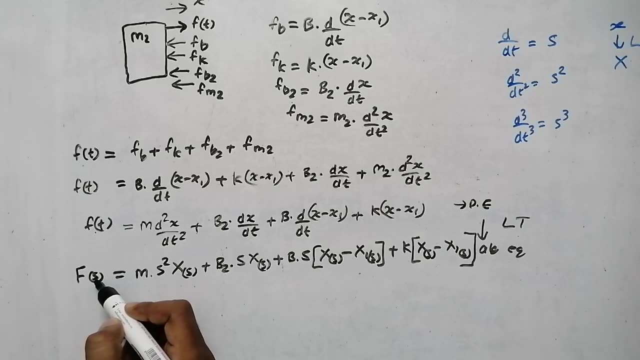 equation using laplace transform. now open the brackets, so this smaller half of t will be converted into capital f of s. okay, in laplace transform, smaller will be converted into capital. okay, so smaller half of t in time domain will be converted into s domain time domain. 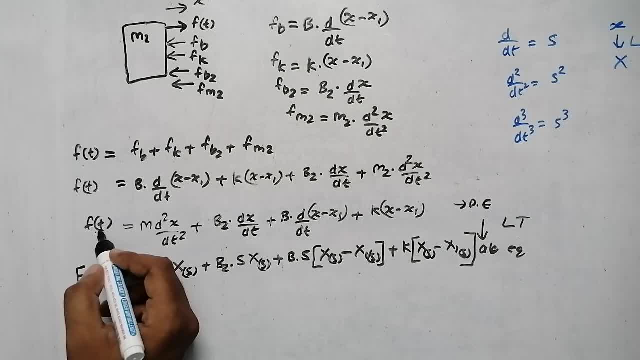 in differential equation. in laplace it is s domain, so smaller half of t conversion into capital f: okay. so that's how you will get this entrepreneurial inequality. Obrigada sa da Renata of s. So capital F of s will be equal to. now we are going to open the bracket, So m s square. 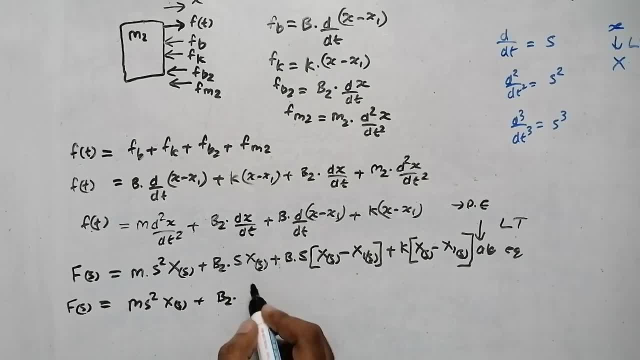 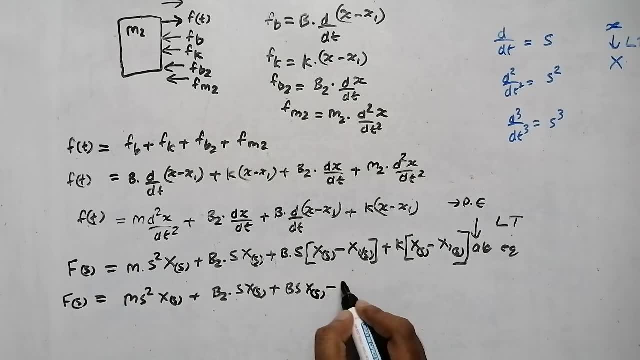 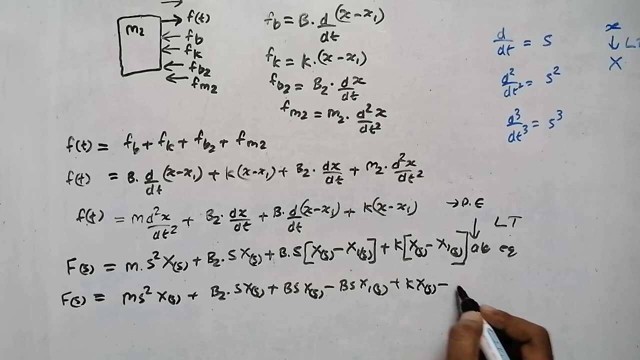 x of s plus b2 into s x of s plus. now open the bracket bs into x of s, minus bs into x1 of s plus opening this bracket it will become k x of s minus k x1 of s. Now x of s is common. 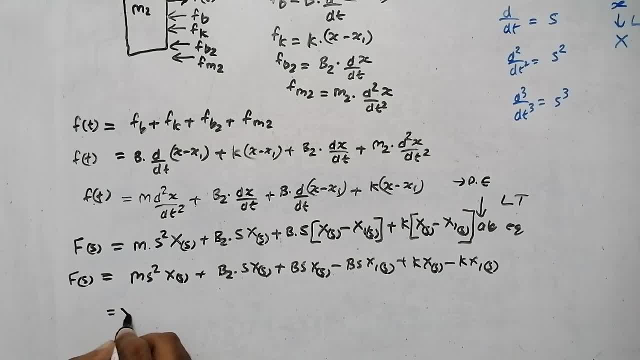 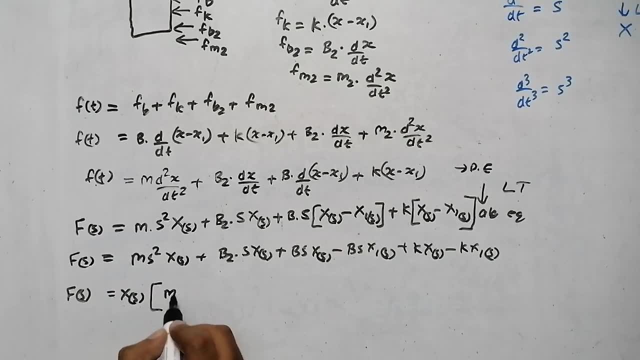 to all this time. So take x of s outside, So it will become x of s. here there is f of s, okay, and x of s I am taking outside. then the remaining time it is m? s square plus b2 into s plus bs, and here we can't take this time because it is x1 and the remaining time it is k. 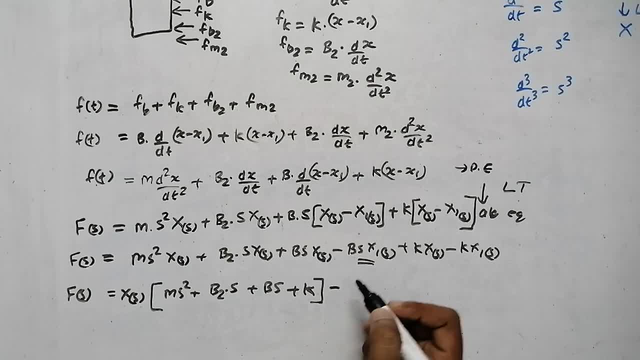 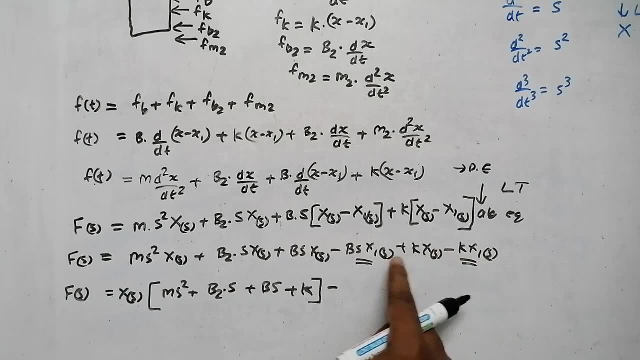 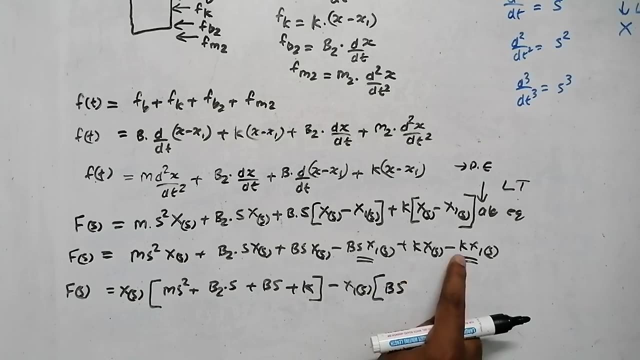 Now close the bracket, then put minus sign. these two are the remaining times minus bs, x1 of s, and here also k, x1 of s. now we are going to take x1 of s outside minus x1 of s outside. then the remaining time it will be bs, and here it is minus k, so minus, and here already I. 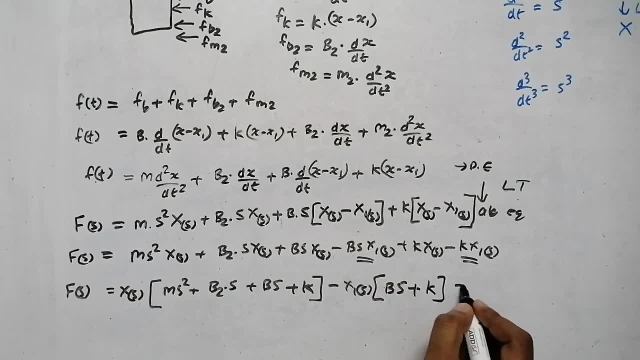 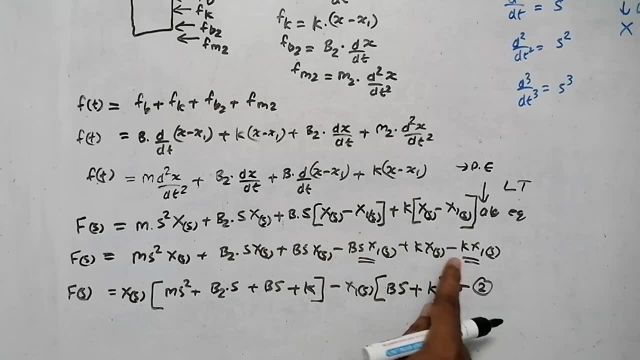 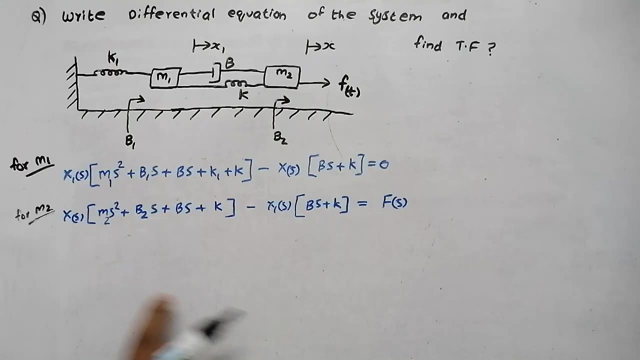 took minus outside so I can write plus, plus k, okay. So this is the equation number two here. both minus sign, so I took minus also outside, then instead it become plus, okay. So this is the equation. Now we got these two equation. Now listen carefully, okay, What do you mean by? 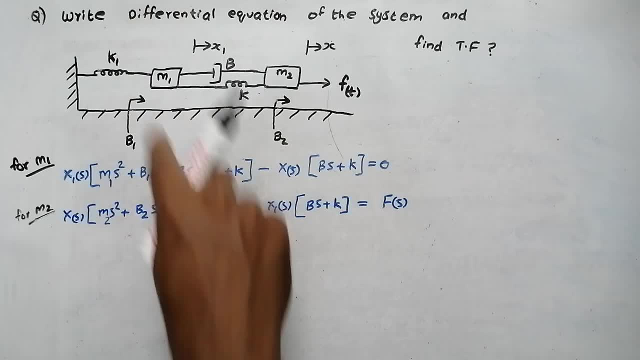 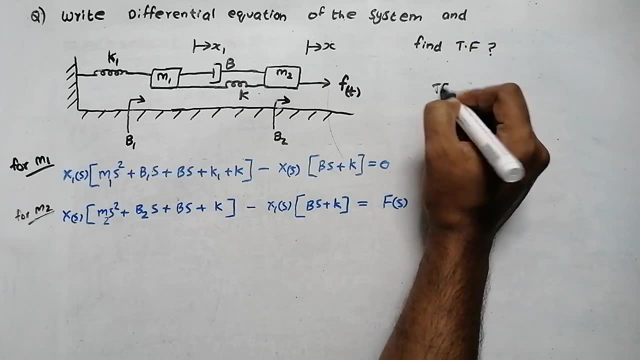 transform. We need to find transfer function. We already found differential equation. From differential equation we converted into algebraic equation using Laplace transform. Now the last step is to find transfer function. So what do you mean by transfer function? It is ratio of output. 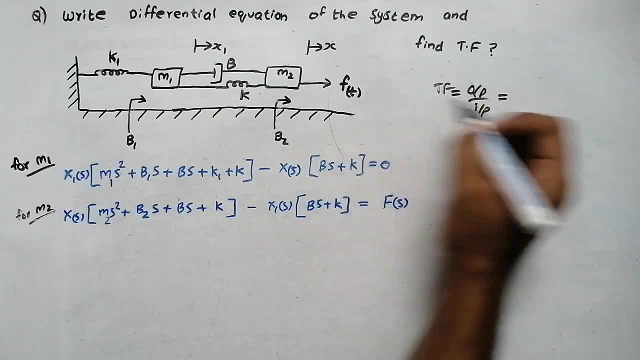 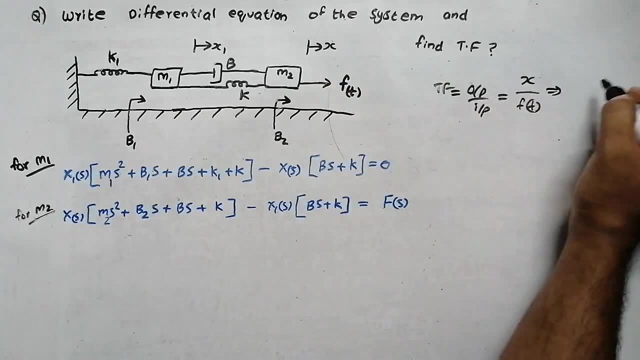 by input Here. what is the input? It is the force f of t, f of t. and what is the output? Output is in Laplace. it will be capital x, x of s in s domain. From time domain, we will convert into x domain. 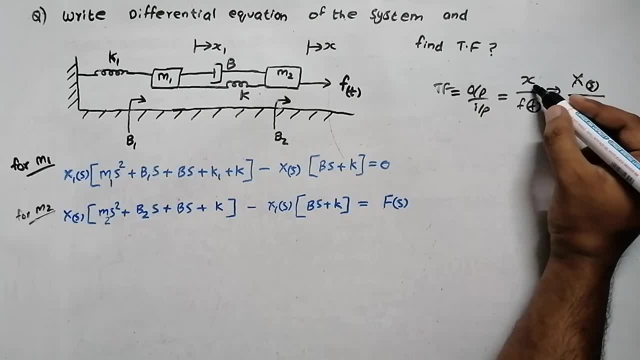 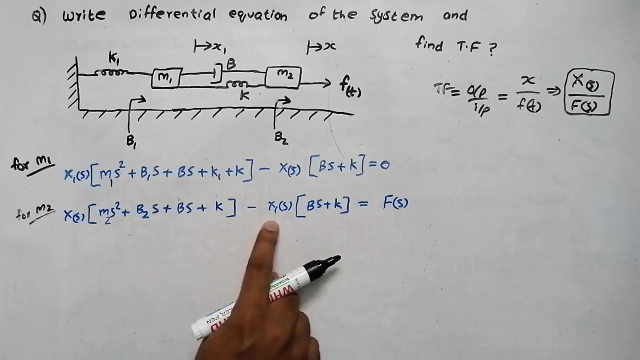 s domain in Laplace transform. So small letter x will be converted into capital x of s. then small letter f of t will be converted into capital f of s. So this is the transfer function that we need to get x of s and f of s. But here we can see x1 of s. We need to remove this x1 of s. Here we have. 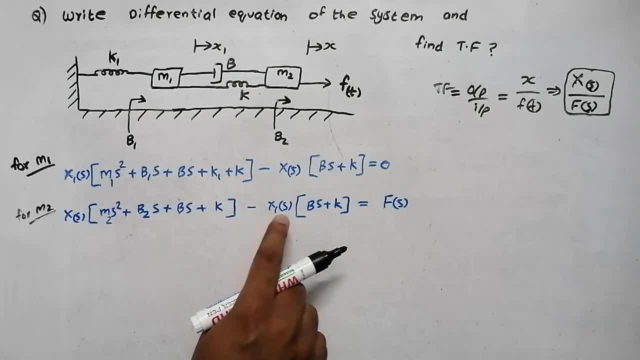 remaining term. So we need to remove this term. How we can remove that From first equation? look at the first equation. okay, From first equation it is equal to 0. So I am going to move this term to the other side, to this side, and what will happen? So, minus going to the opposite after. 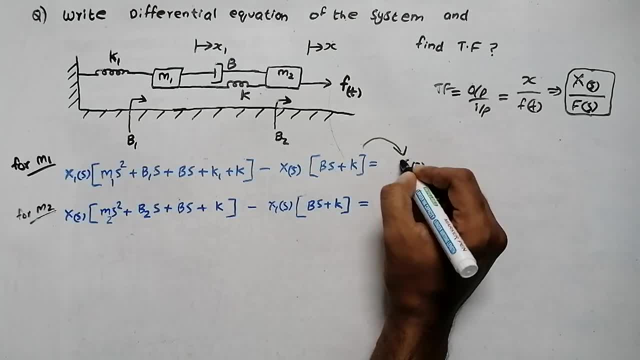 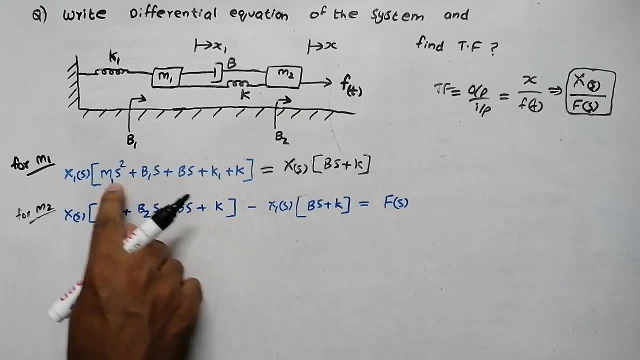 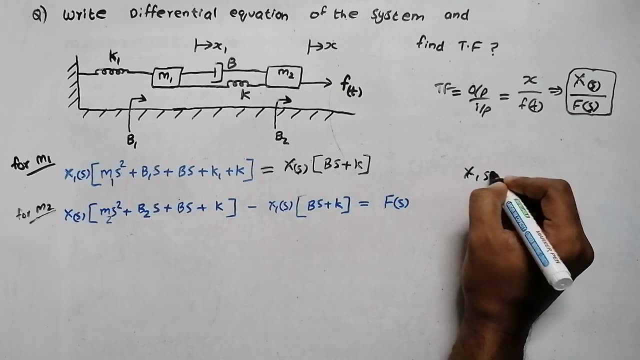 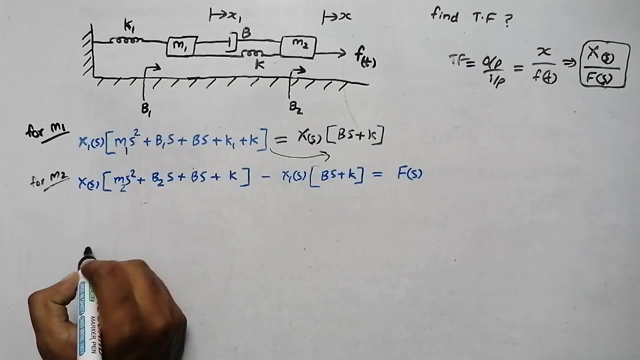 equal to sign, it will become plus. So it will become x of s, then bs plus k. So from the first equation I got like this: Now I can write x1 of s, okay, So x1 of s will be moving this term to the denominator. That means x1 of s I am keeping here. then put equal to, then 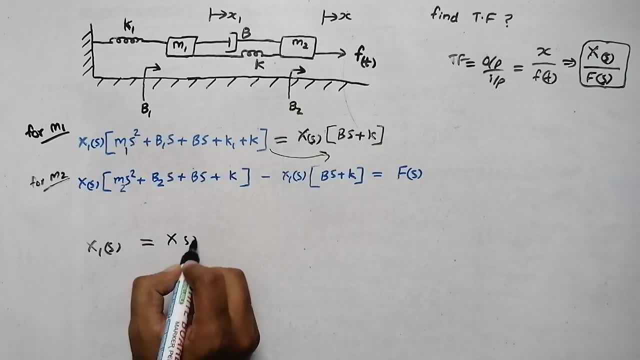 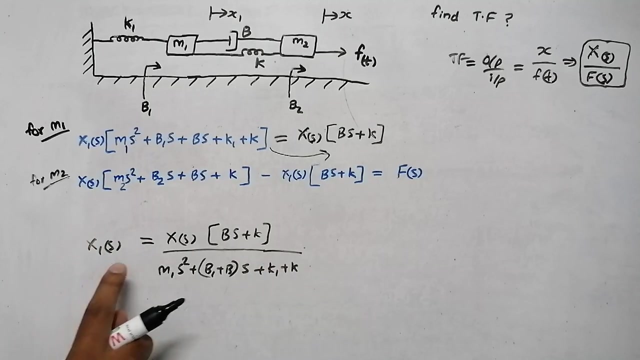 I am going to move this term to the denominator side, So x of s into bs plus k. divided by all this term, okay, That is m1 s square plus here s is common. So I am going to write b1 plus b into s plus k1 plus k. So this is the value of x1 of s. Now substitute this x1 of s. 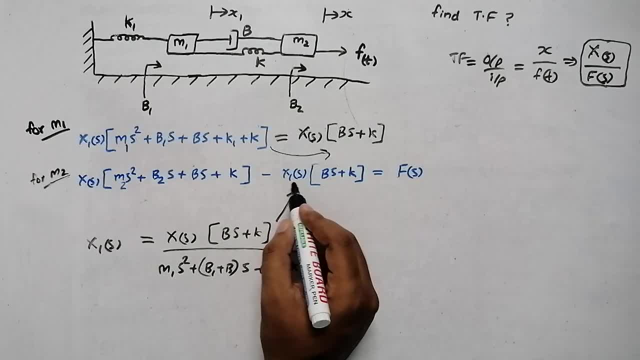 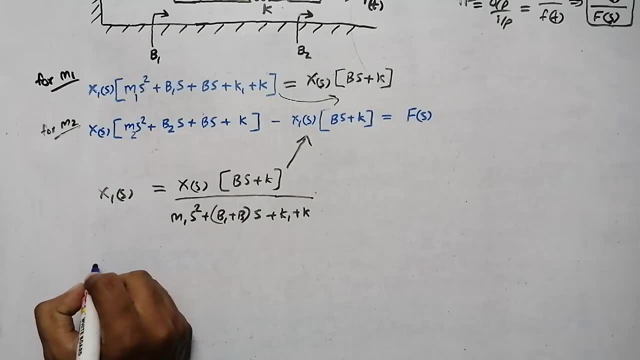 here. Here we can see x1 of s right in the second equation. So for x1 of s, substitute this term here. So I am going to write the second equation. Second equation is this one, that is x of s, then m2 s square. 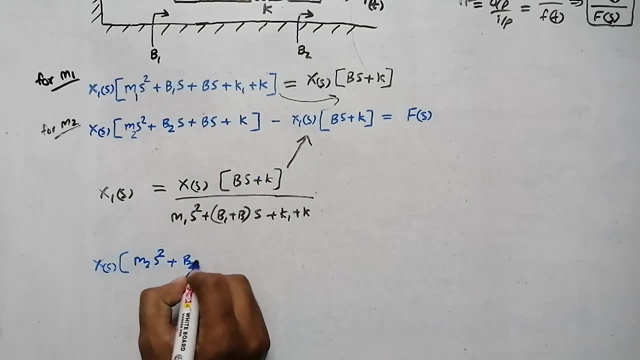 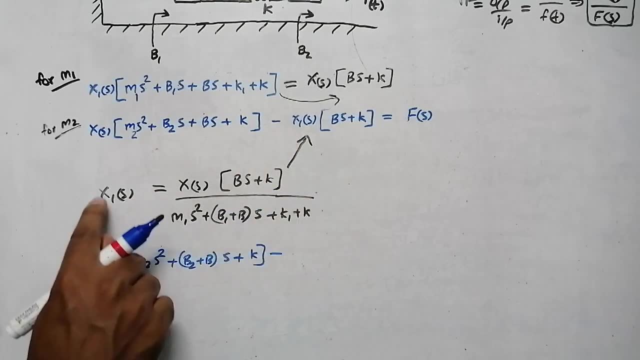 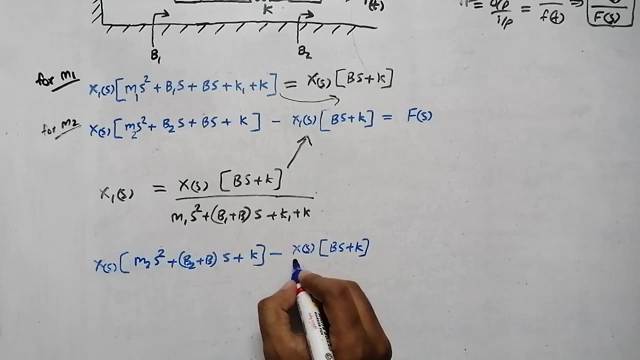 plus here s is common, So I am going to write it as b2 plus b into s plus k minus x1 of s. Instead of x1 of s. I am going to write this term, that is, x of s into bs plus k divided by m1 s square. 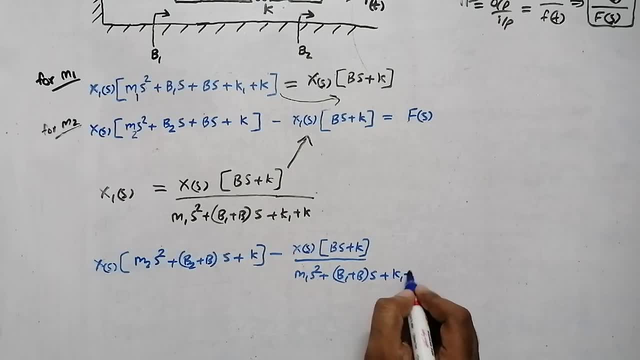 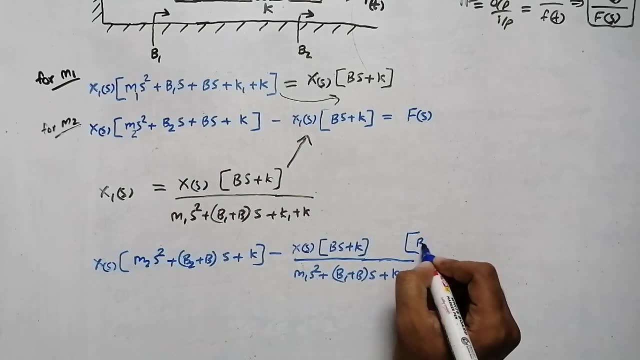 b1 plus bs plus k1 plus k. Okay, instead of this x1 of s, I wrote this thing In the remaining time it is bs plus k. So after x1 of s, the remaining time it is bs plus k. That is equal to f of s. 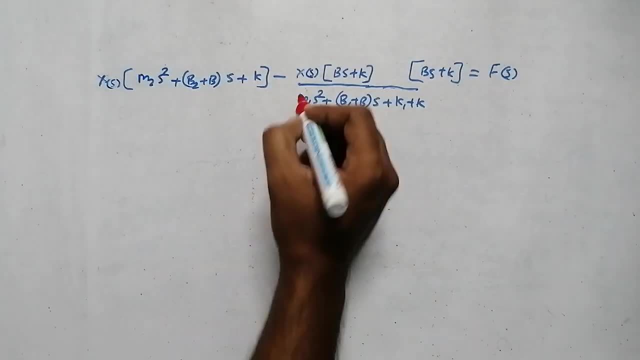 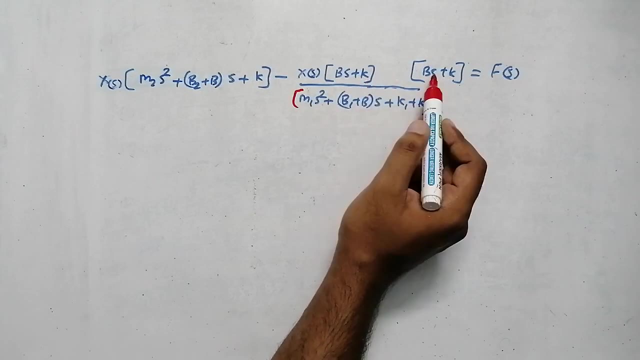 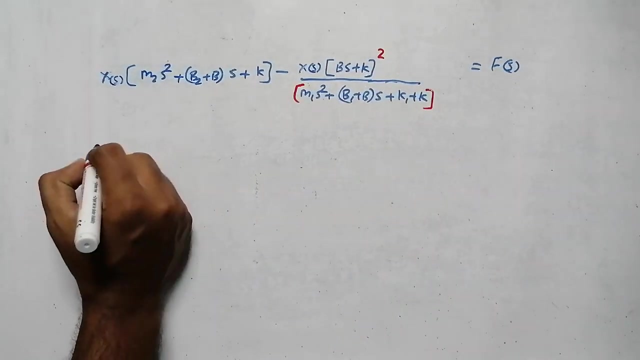 Now there is only a substitution part. Listen carefully, okay. So this is a denominator and here it is a numerator. and here, bs plus k, bs plus k, x into x, We will write x square. So bs plus k into bs plus k, we will write bs plus k square. Listen carefully, okay. So first of all, 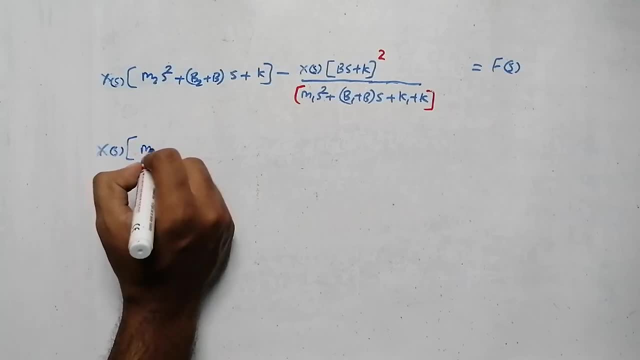 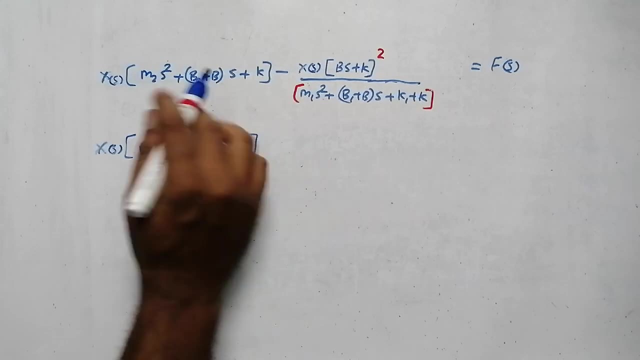 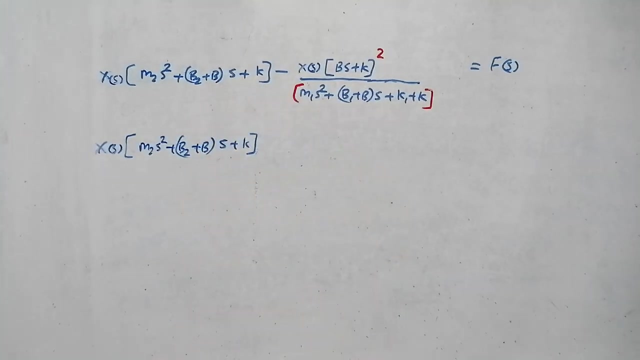 we will write this term, that is x of s into m2 s square plus b2 plus b into s plus k. Now, this was in the numerator side. Now we are going to cross, multiply it. okay, Then it will become multiplied by the remaining time. is the denominator. So we will write the denominator. it is m1 s square plus. 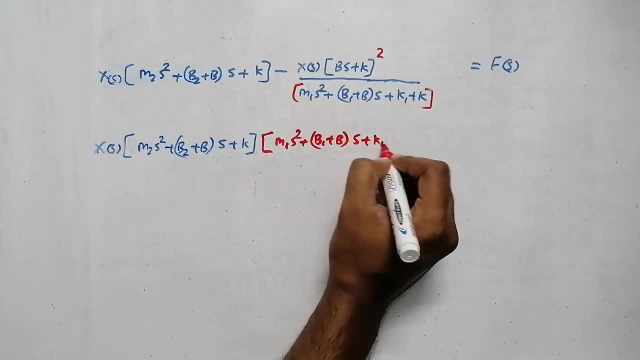 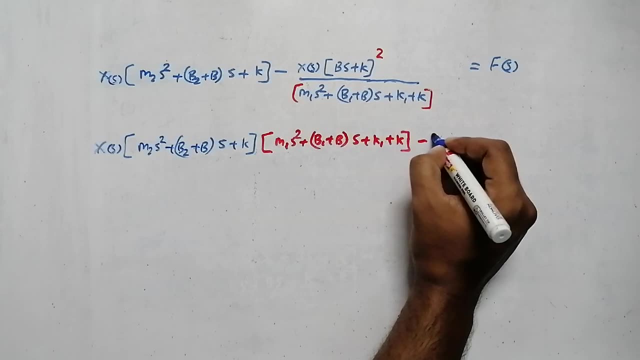 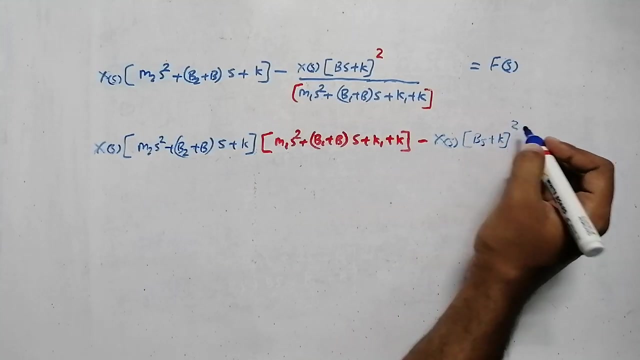 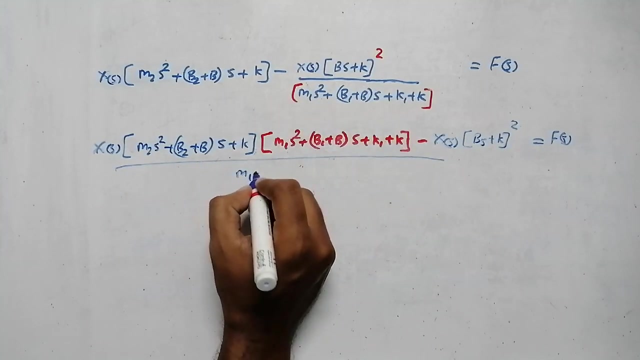 b1 plus b into s plus k1 plus k. That was the denominator. Then the remaining time it is minus x of s, x of s bs plus k, the all square That will be equal to f of s, Now all divided by our denominator Denominator, it is m1 s square plus b1 plus b into s plus. 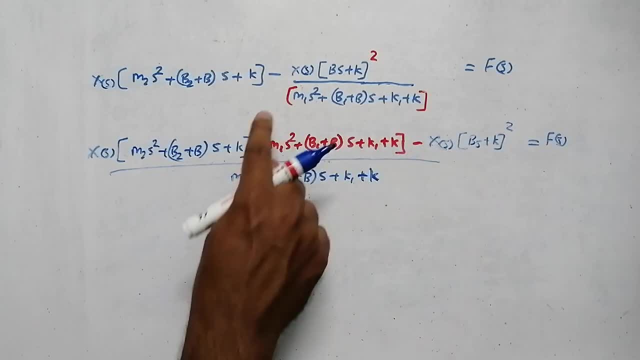 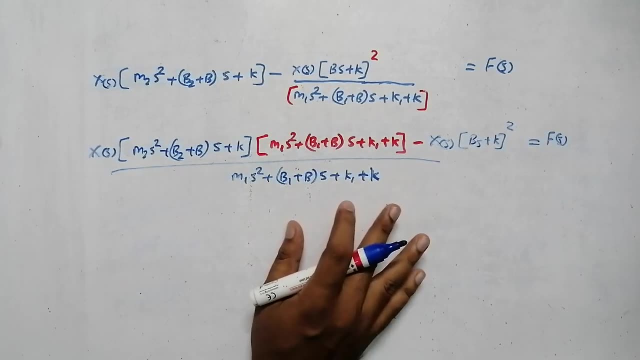 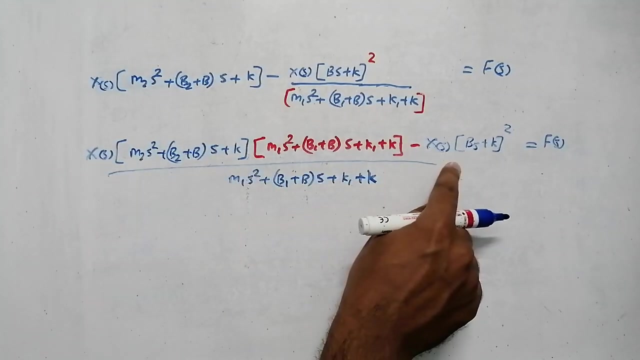 k1 plus k. okay, Here, this was in the denominator. We just cross, multiplied it, Then the denominator, we wrote like that itself. Now what we need, as we can see here, x of s is common to both these terms. okay, Here x of s is there. Here x of s is there. So we are going to take x of s. 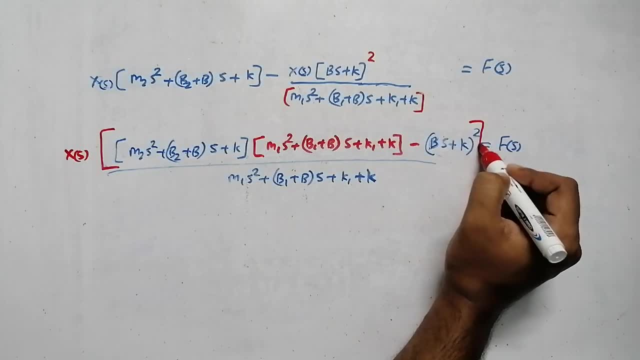 outside. So I took x of s. x of s was common to both this term, So I took x of s, x of s, x of s outside. Now I got x of s and f of s. So my transfer function is ratio of x of s by f of s. 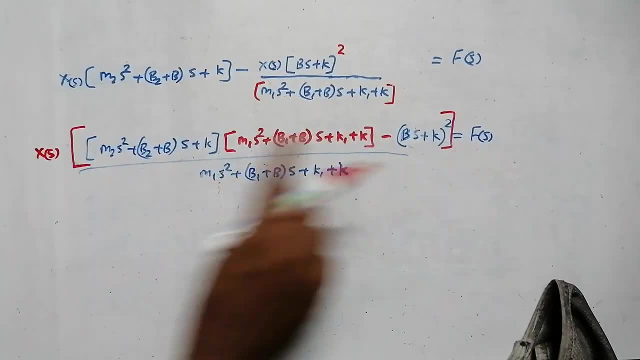 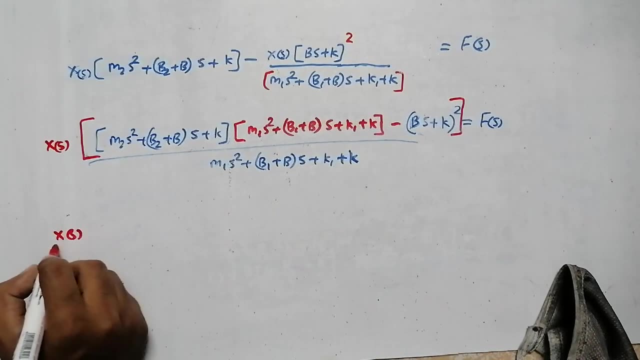 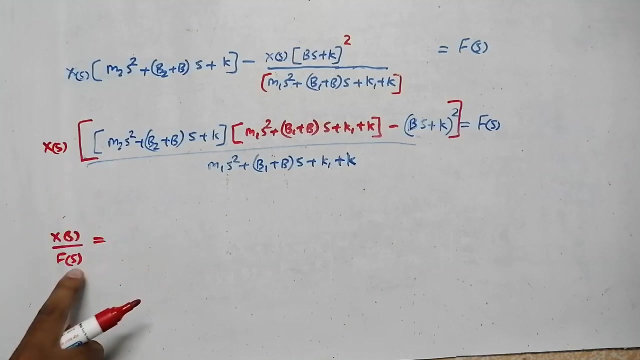 So x of s by f of s. So, keeping x of s here, I need to bring f of s in the denominator side, That is, x of s divided by f of s. okay, So I need to move this to the other side, the numerator side. 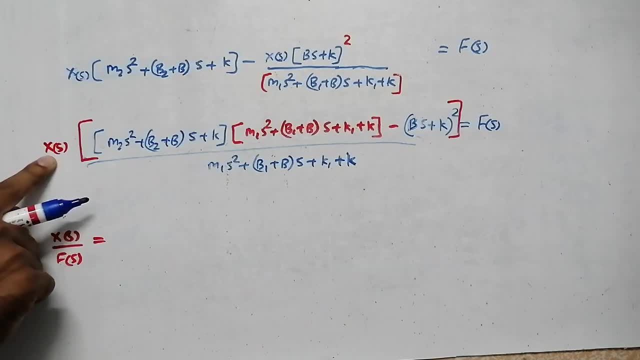 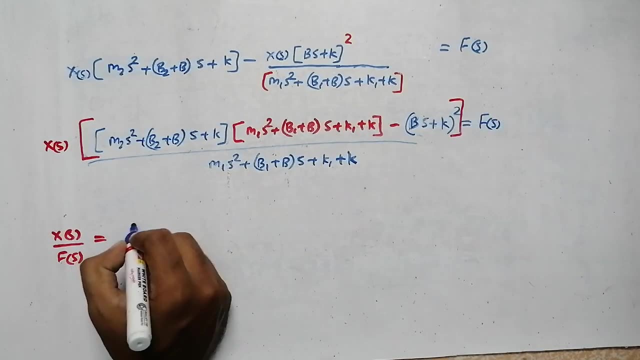 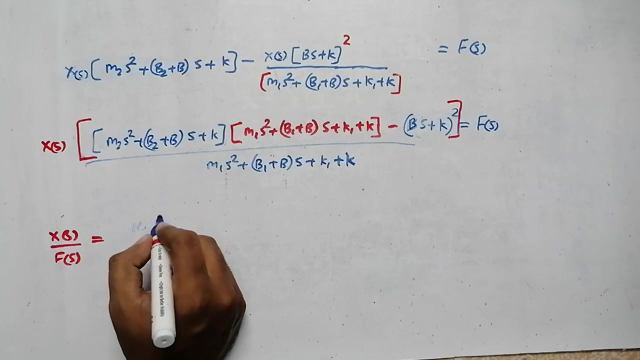 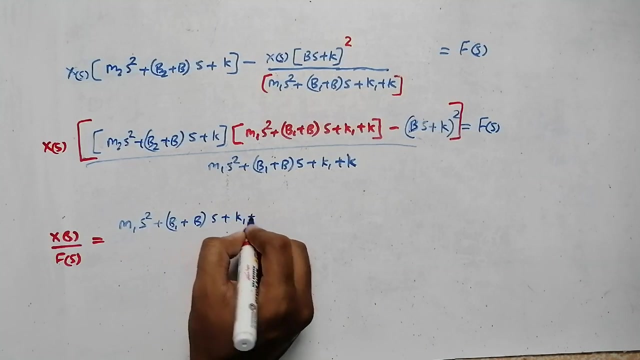 So it will become x of s I kept here, Then f of s. I bring here Then this denominator I need to put in that side, So it will become. it will become the numerator. Here it is denominator, There it will become numerator. So m1 s square plus b1 plus b, s plus k1 plus k, divided by all this.